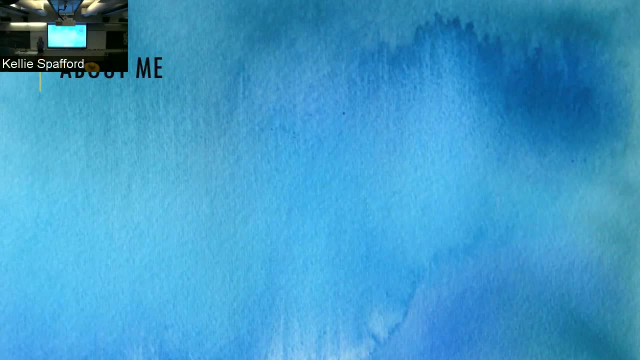 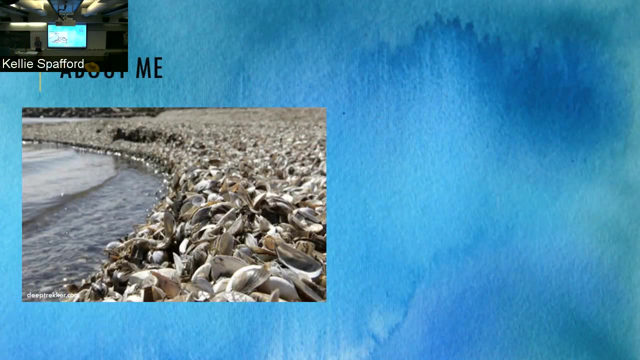 But then, as I grew older, I also developed an awareness for changes that were occurring to these environments that I had loved so much. The first of these was the invasion of zebra mussels. So zebra mussels are a type of animal that is very sensitive to the environment. 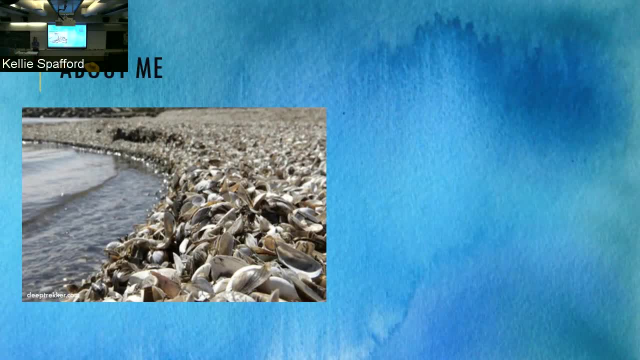 So zebra mussels are a type of animal that is very sensitive to the environment, And so the first of these was the invasion of zebra mussels, And so the first of these was the invasion of zebra mussels. There are different, prettiest, different type of freshwater shellfish that are native to Ukraine and Russia. 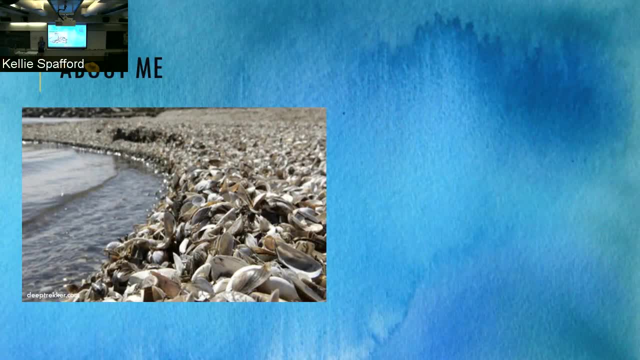 and invaded the Great Lakes region around the 1980s, but really started to proliferate during my childhood, And changes I began to notice were once they'd become more vanquished with these mussels and, in then, boat hulls and intake pipes. 5. 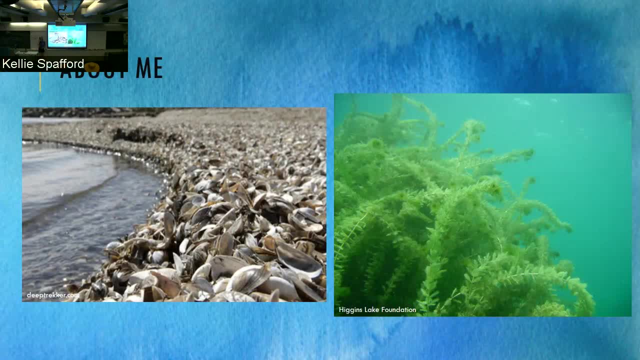 koosta actually distinguish the two origins. So this is one change I noticed. and another changed was the invasion of Eurasian milfoil. eurasian milfoil 3: 1 Europe and North Africa, but started to proliferate in the Great Lakes region around the 2000s. 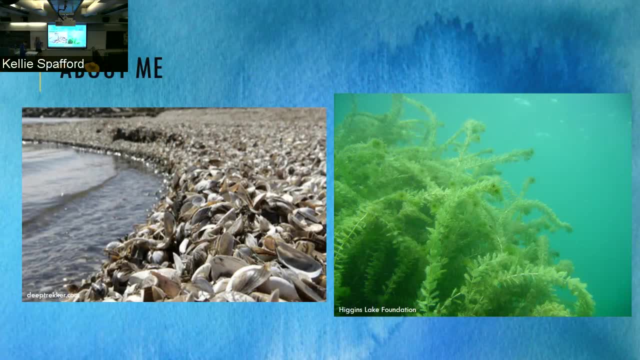 So a change I noticed associated with this was these large, dense mats being formed by this alga and kind of really impacting the ecosystems it invaded. So these are really big problems in the Great Lakes region during my childhood and currently still are. So I became really concerned with why these changes were happening to these ecosystems. 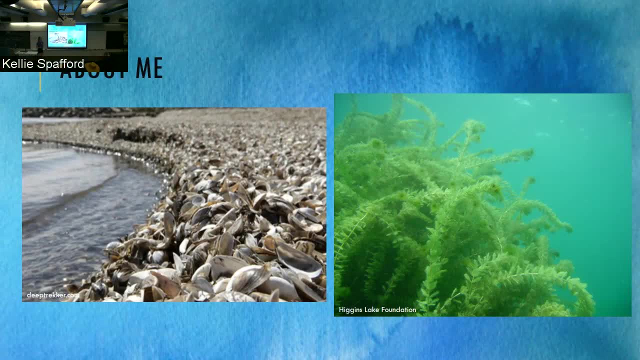 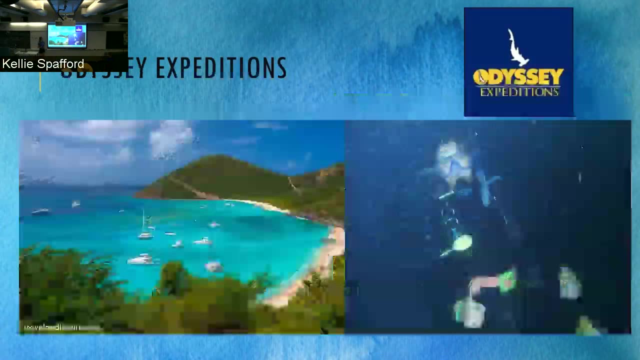 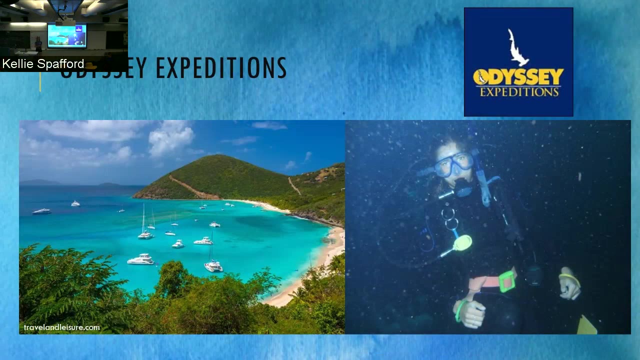 I love so much, but also how they could be fixed. So this was kind of my first step towards conservation and conservation of these aquatic communities that I love so much. So this led me to a particularly transformative experience with this program called Odyssey Expeditions, which basically leads high school and middle school age students on sailing. 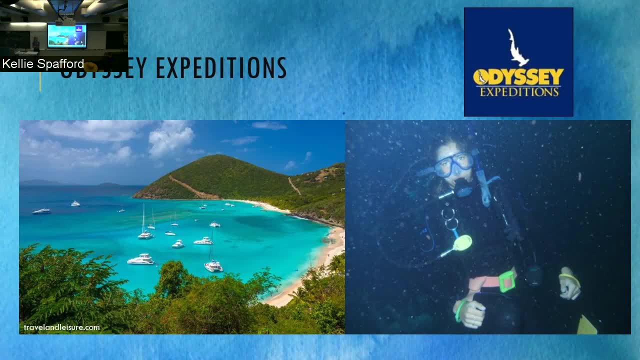 trips throughout the Caribbean And teaches them about the ocean environment but also conservation issues associated with the ocean. So during my time with Odyssey, I learned how to sail, I got SCUBA certified, I got my open water and advanced certifications. 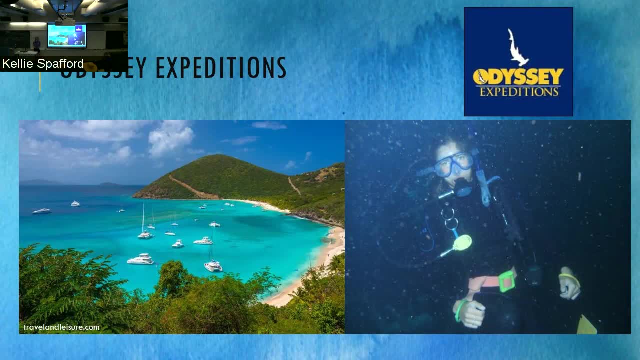 And then I also got my first taste of underwater science. So I learned how researchers rehabilitate sick or injured sea turtles and kind of eventually be able to reintroduce them into the wild. And then I also learned- Or I probably should say I learned- how to reintroduce them into the wild. 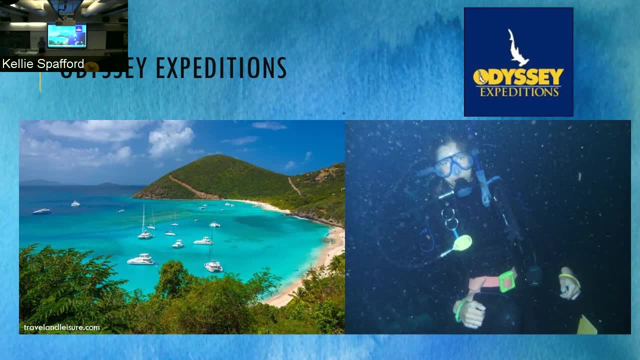 And then I participated in my first underwater survey So I actually got to ID and count reef fish that were included in that year's population census. So after participating with Odyssey I was pretty convinced that marine ecology and marine conservation was something that I wanted to pursue on a future career. 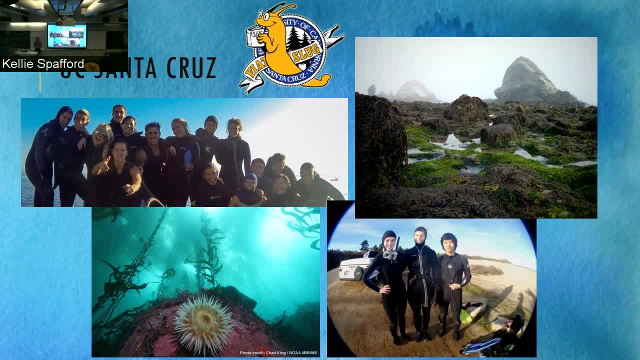 So then I started to pursue a degree in marine biology from UC Santa Cruz, And I got my scientific diving certification from UC Santa Cruz, Which basically allowed me to conduct underwater research on my own And then also expand my knowledge base of the ocean with classes like marine conservation. 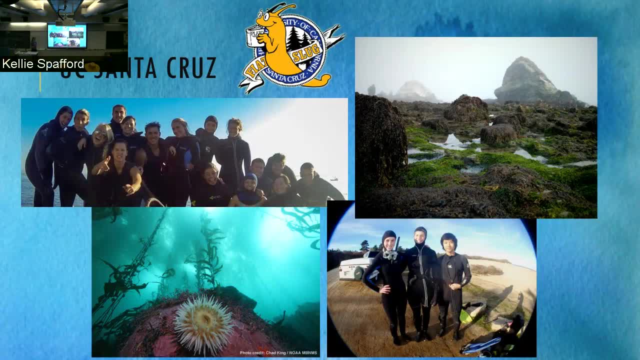 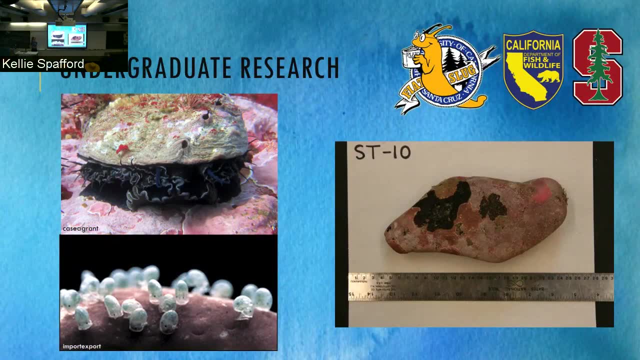 kelp, forest ecology and marine botany. And in addition to these classes I was taking, I was also lucky enough to participate in several research projects. The most notable of these was dealing with abalone conservation. So abalone is a type of marine mollusk. 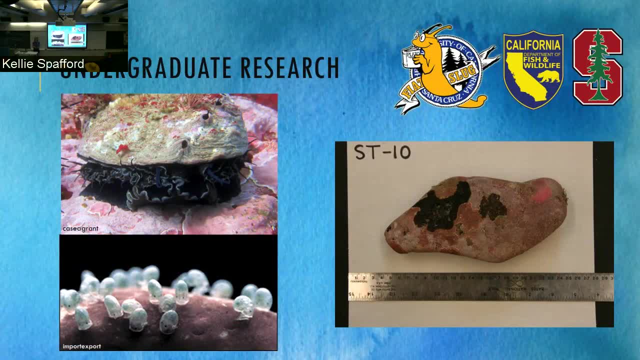 And along the West Coast there are actually several species of abalone that are found in the ocean, And so that's kind of the first thing I learned about marine conservation. So there's actually several species, many of which are unfortunately threatened due to overfishing and disease. 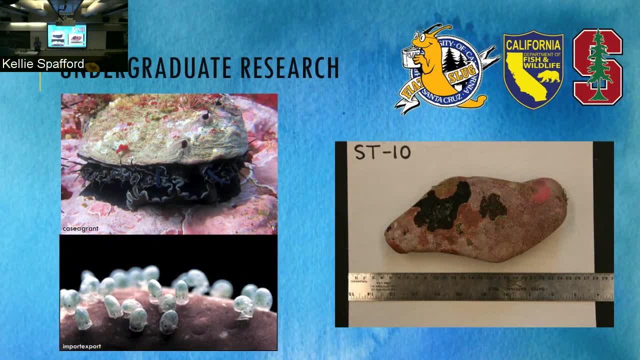 So the project I was associated with was looking at methods that would try and try to restore these populations back to their natural levels. So abalone is pretty cool because it has a larval stage that basically floats around in the water column and requires this pink, pink like looking algae called crustosaccharum. 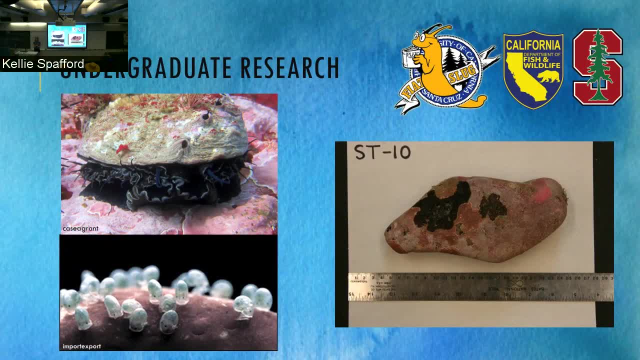 algae to initiate this process, initiate its settlement from the water column onto this alga and then from there it initiates the transformation into the adult stage. So this algae plays a really important role in its like this, enabling life history, but little is really known about 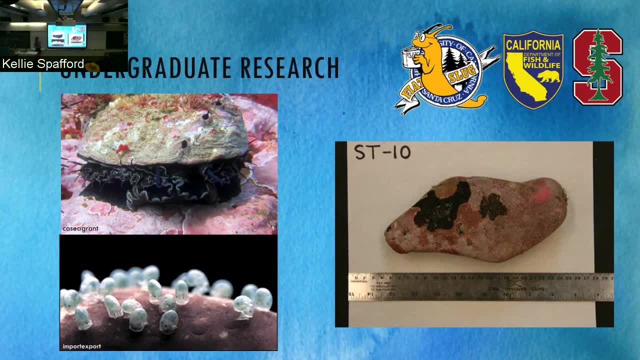 why are the ecology of this algae. So my role was to look at many, many cobbles with this algae growing on it and try and tease apart morphological groupings of this algae, because it's really hard to distinguish this algae to the species level and see whether there are more or less abalone larva. 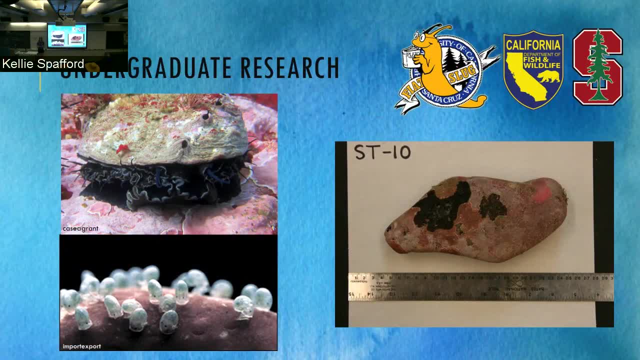 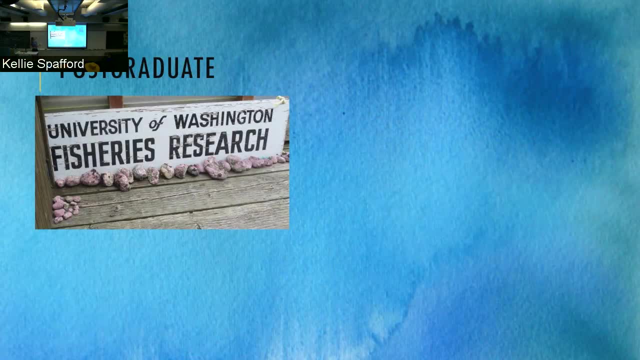 settled on these different groupings to see if there is some type of preference associated with this algae. So following undergrad, I continued on working with this abalone project and so I went up to the University of Washington with some- the Department of Fish and Wildlife, looking specifically at 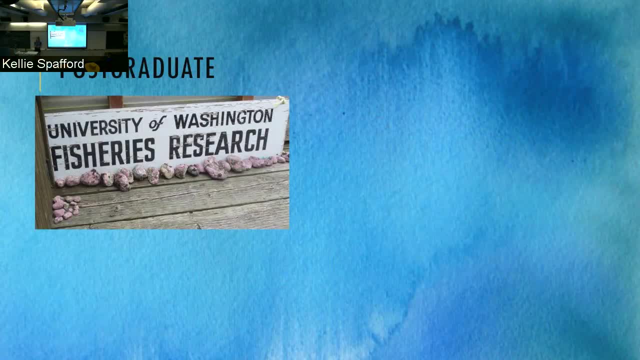 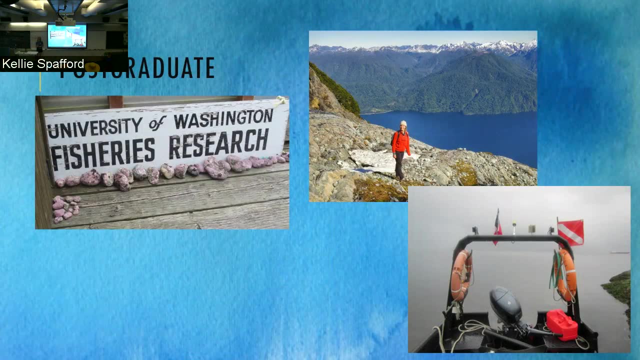 how this algae influenced populations of pinto abalone in the San Juan Islands. And then I started working down at a research station in Chilean Patagonia for a couple of months. and then I got a job with the Department of Fish and Wildlife, with the ground fish ecosystem. 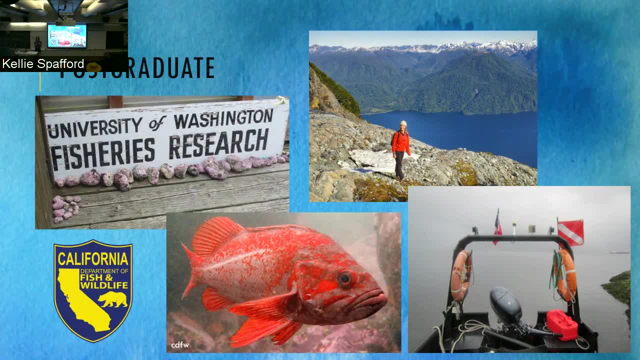 Basically, my main role with these guys was helping with their outreach and talking to fishermen and making sure they understood the ground fish fishery. So this was about a year post-graduate and I was testing the waters in a variety of different ways and I figured that I wanted to continue my education. 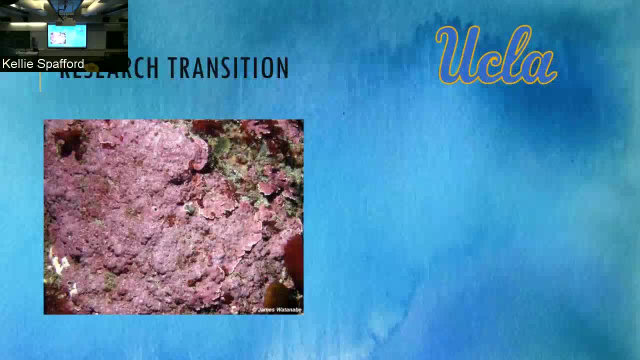 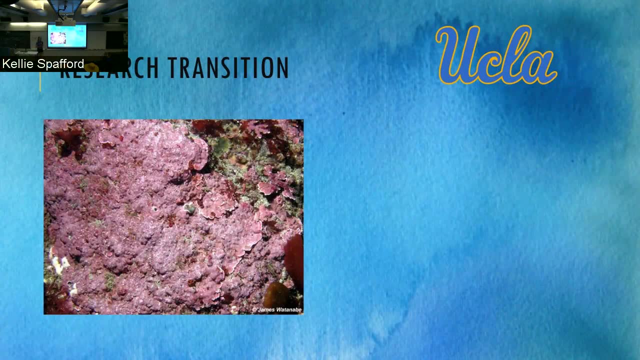 with a graduate degree. So I started a PhD at UCLA and was pretty set on continuing my work with this crustacean, coral algae and abalone. But as I started to delve a little bit deeper into it I realized that a lot of the work I would be probably doing for my dissertation would be 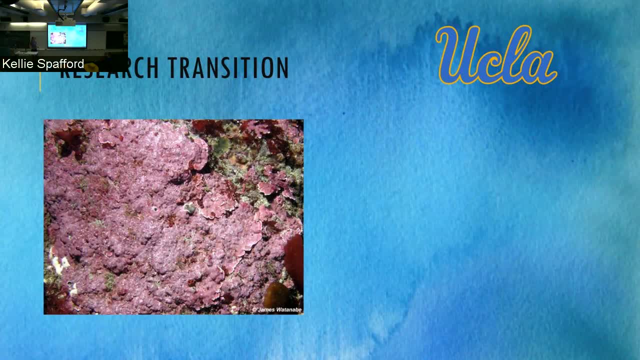 baseline descriptions of the ecology of this algae, which is important, but didn't really have the applied conservation aspect that I really wanted. So kind of trying to figure out what I want to do. next I came out to Catalina Island as a teaching assistant for a field quarter and started to learn about the sargassum coronary invasion and how it was potentially 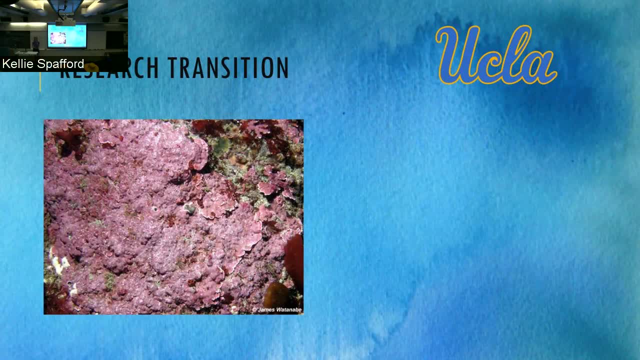 impacting the ecosystem, but also how little was still known about what it was doing out here and also why it was so successful. So I made the transition from one charismatic macro algae to the next and I started studying sargassum coral algae. 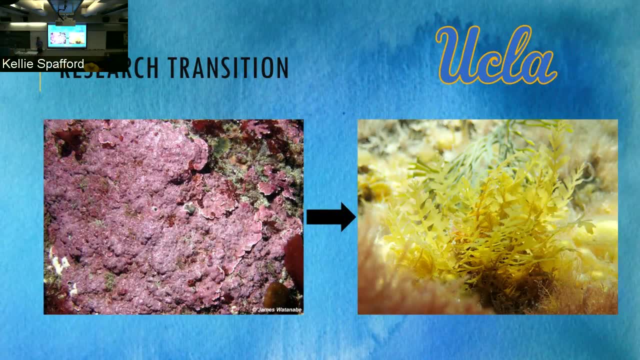 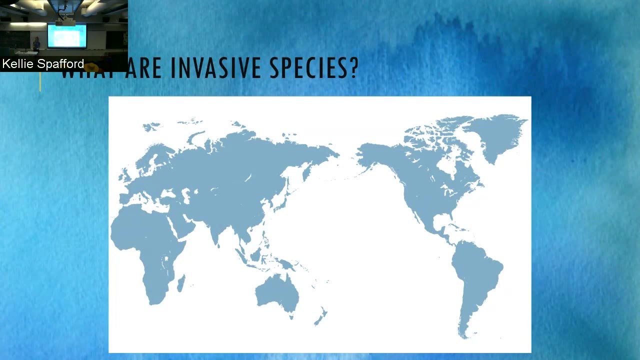 Which is where I am now. So before I get into the details of my research, I wanted to get a little bit of a background that kind of informs what I'm doing now. So what are invasive species? While many species may travel from their native location to a non-native range through a variety of vectors, 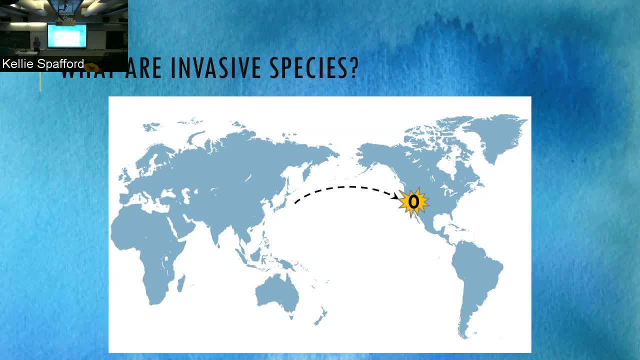 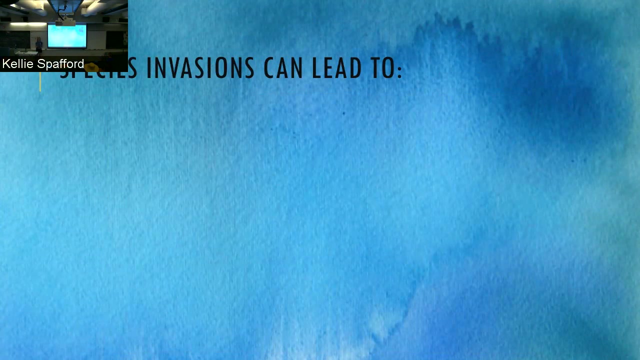 species that have really no discernible impact on the environments they invade are considered to be introduced species. On the other hand, species that have a negative impact on the environment they invade are considered to be invasive. So species invasions can lead to a variety of negative impacts, including. 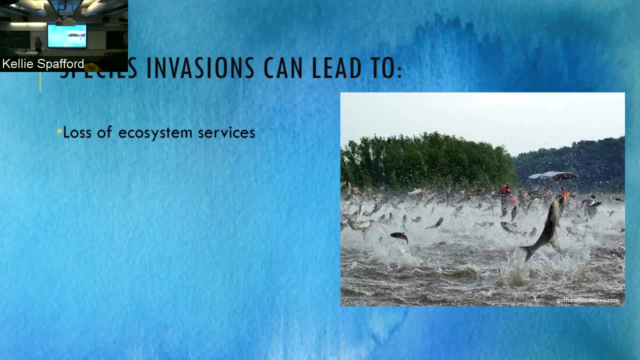 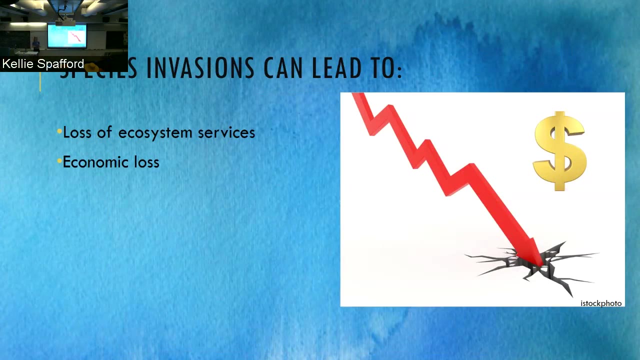 loss of ecosystem services, or basically the services the ecosystem provides to humans, such as food, recreation, such as boating, fishing, etc. And because of the loss of these ecosystem services, invasive species can also lead to economic loss, because these ecosystem services often generate. 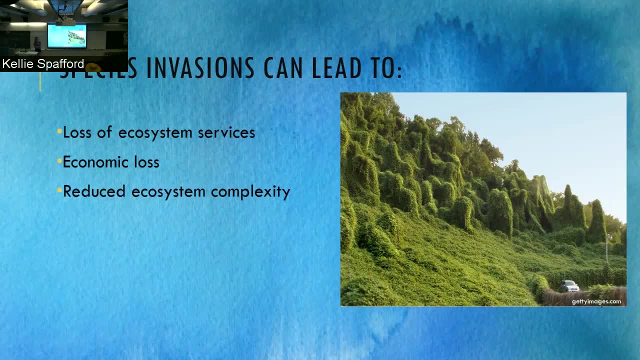 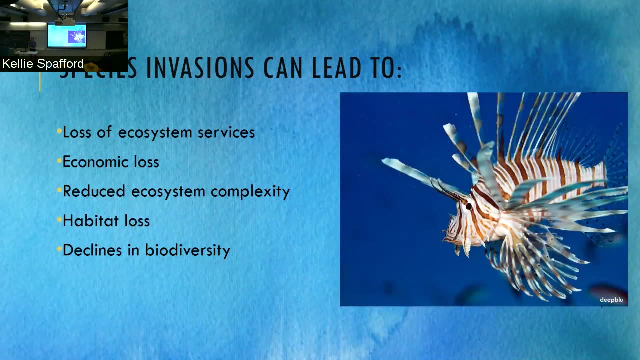 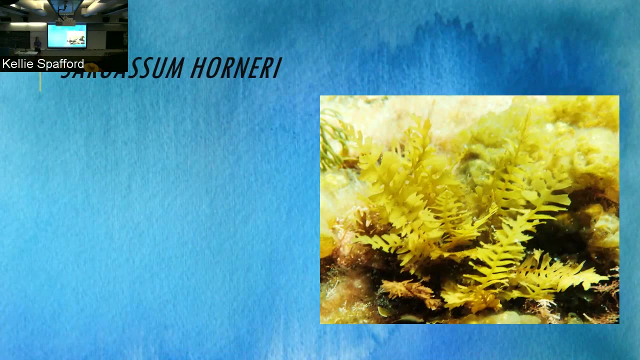 a high type of revenue. Additionally, species invasions can lead to reduced ecosystem complexity, habitat loss and, because of these issues, they can also lead to severe declines of biodiversity. So a little bit transitioning to my study species: Sargassum porneri. 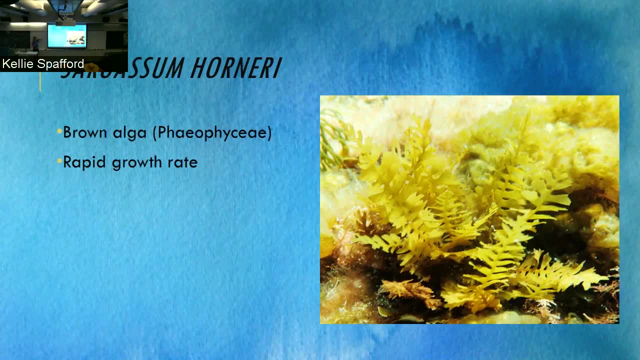 It's a brown alga in the class Phaeophyciae. It exhibits a rapid growth rate and a high fecundity, so it's able to produce many baby sargassum pretty quickly. It can grow up to three meters in length, so it's capable of forming these dense canopies that. 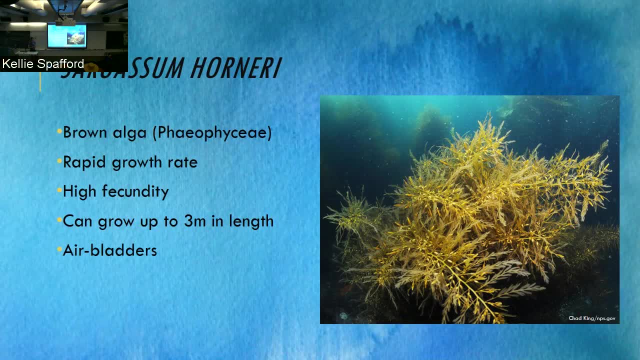 create a really shaded environment in the understory. It possesses air bladders that buoy the individual up towards the light and also, when it becomes attached, it's able to kind of float long distances that facilitate long-distance dispersal. It has a high temperature tolerance and an annual life history, so it completes the entire life cycle within one year. 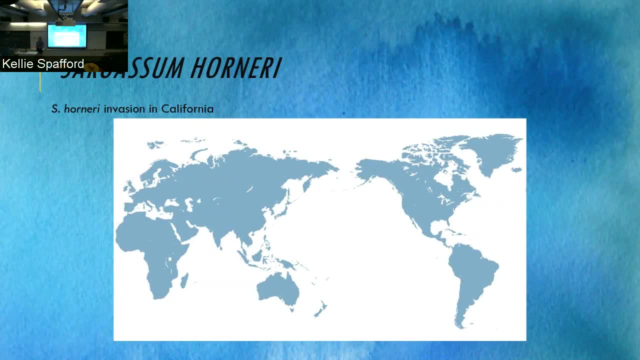 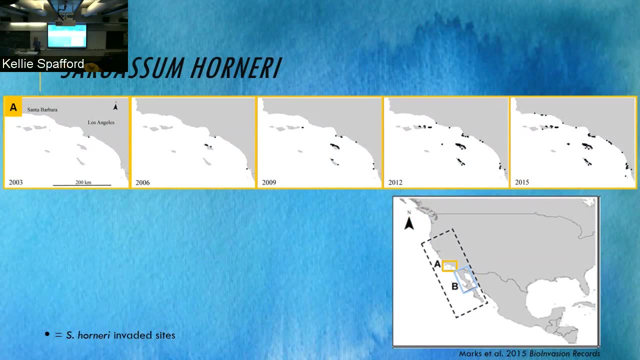 So Sargassum porneri is native to Korea and Japan and it arrived in Long Beach Harbor in 2003.. Since its arrival it has spread throughout Southern California, so throughout the Channel Islands, and then north towards Point Conception. 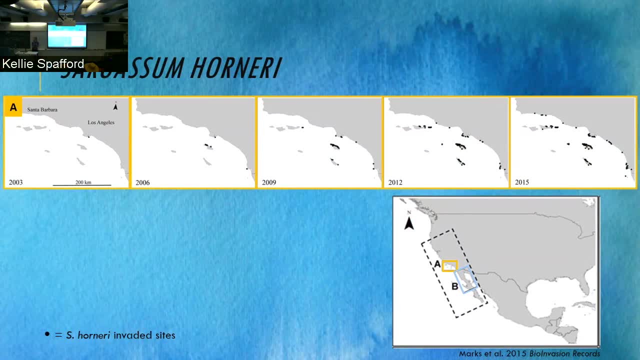 these little dots represent Sargassum porneri abated sites, and then also it's spread south into Baja California. So despite its rapid proliferation and widespread range, little is known really about why it's so popular, and it's also not just about the species and the environment. 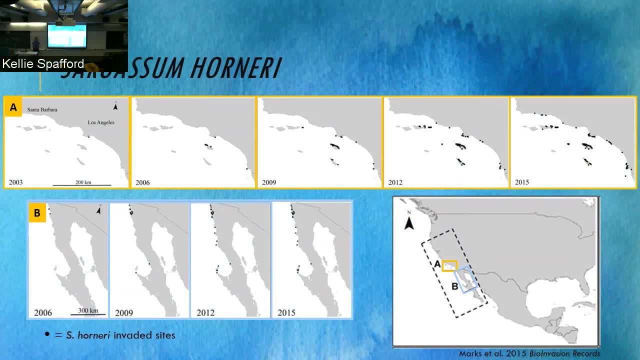 why Sargassum horneri is so successful versus other introduced species and whether certain communities are more susceptible than others. So, where Sargassum horneri is able to establish, it's capable of forming these dense monocultures that are hypothesized to be out-competing native. 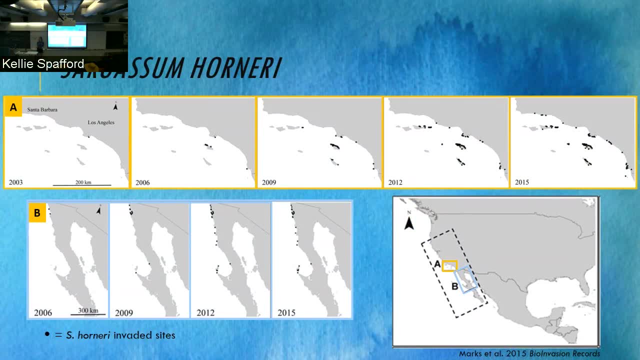 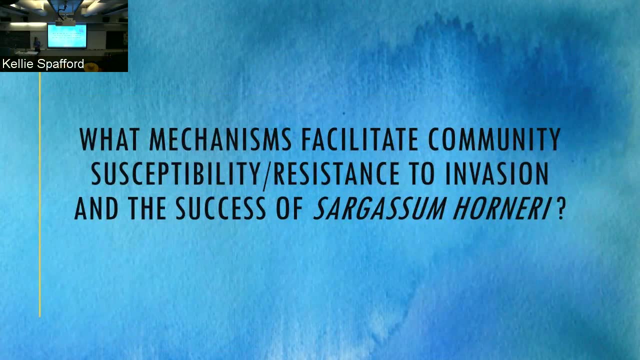 algae for space and light which can have potentially severe impacts on the ecosystem. So this kind of leads me to my research question, which is what mechanisms facilitate community susceptibility or resistance to invasion and then also facilitate the success of Sargassum horneri? 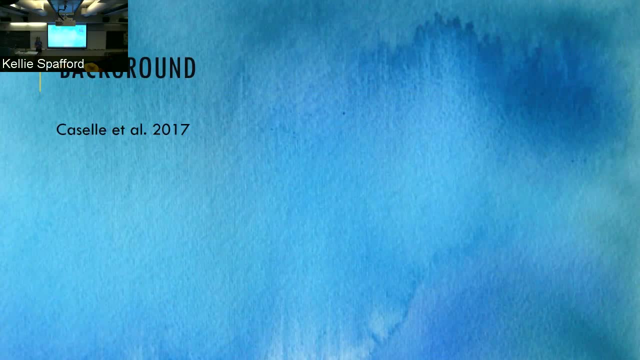 So a little bit of background behind this question. Recent research actually found that, from studying long-term data, that there are communities that are more or less susceptible to invasion. So these, yeah, as I mentioned, are conclusions from long-term data, from the 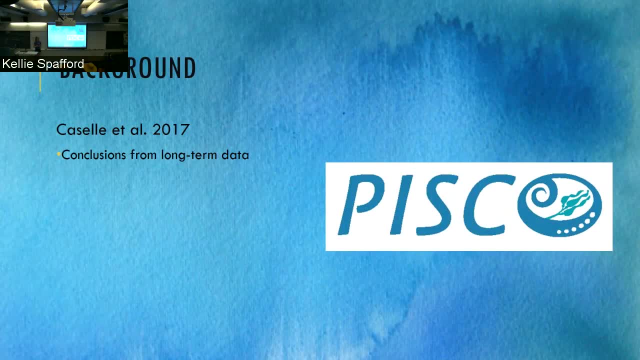 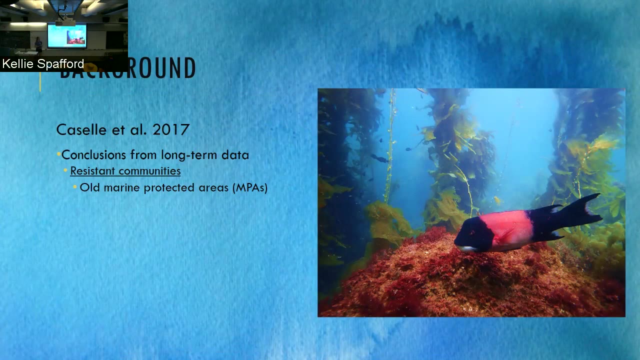 northern Channel Islands, which is basically kind of community ecology data, And what they found was that resistant communities were those that had been protected from fishing for a long time, so older marine protected areas or MPAs. So in these sites there was a high abundance of these top predators. 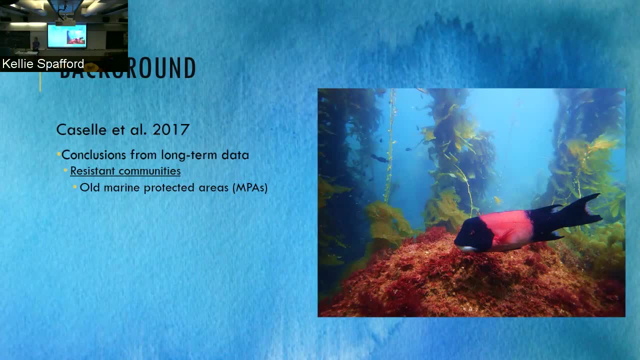 California sheephead, pictured here, and then California spiny lobster, because they weren't being overfished, because they were protected. And these predators? they really like to eat sea urchins, which, in turn, are voracious herbivores of algae. 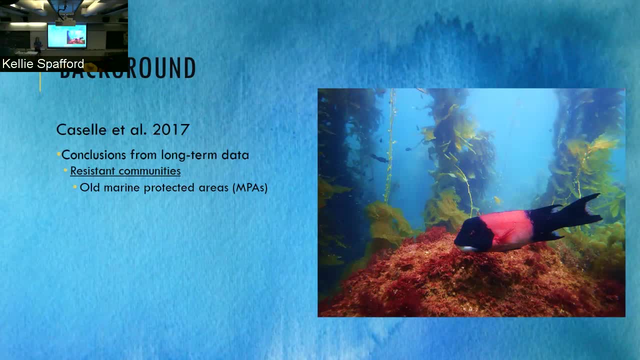 So in these sites that were protected, these abundant predators were able to keep sea urchins under control and in turn there was a diverse algal community in these sites. So when Sargassum horneri, when they predicted where Sargassum horneri was trying to invade, 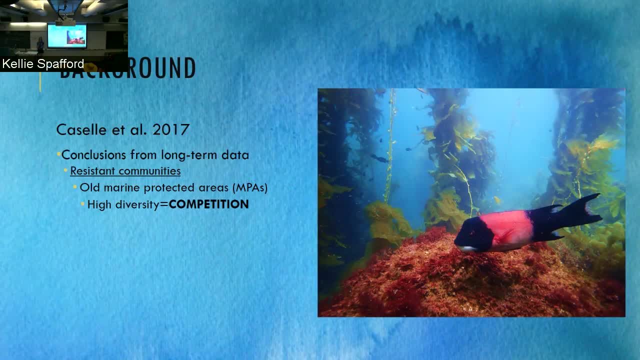 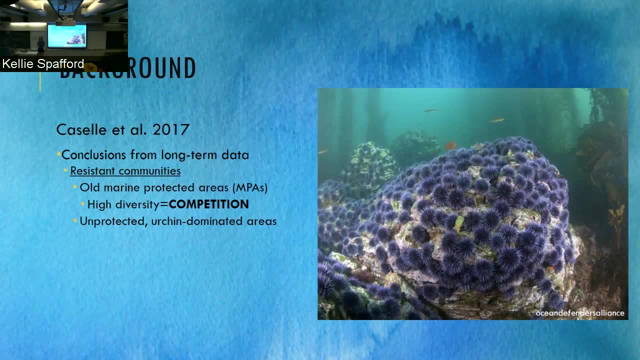 this diverse algal community was out-competing Sargassum horneri, and Sargassum horneri was not able to. On the other hand, these researchers also found that sites that were unprotected from fishing were also resistant to invasion. So in these sites, sheephead and lobster were overfished. 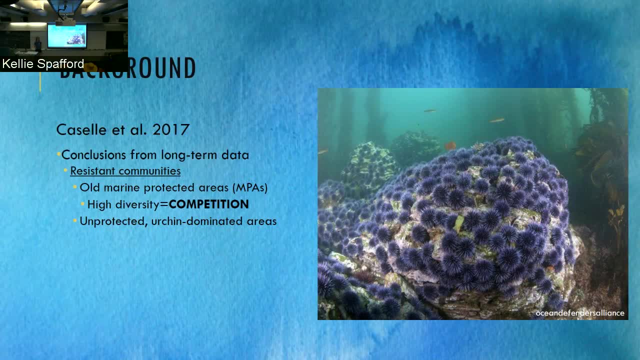 and because of that urchin populations were overly abundant. And because of these overly abundant urchin populations, the algal community was decimated, including Sargassum horneri, which is based on these predictions, So these were also resistant to invasion. 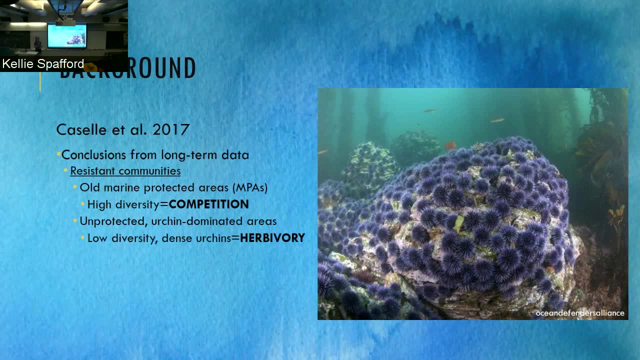 not because of a diverse algal community but because of intense herbivory pressure. So herbivory was a mechanism for controlling Sargassum horneri there. And then the researchers found, or predicted, that the most vulnerable communities were: 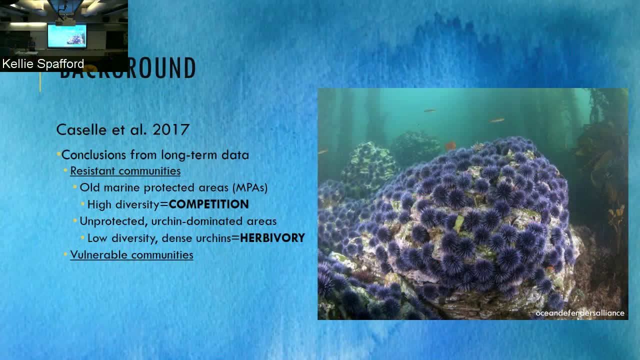 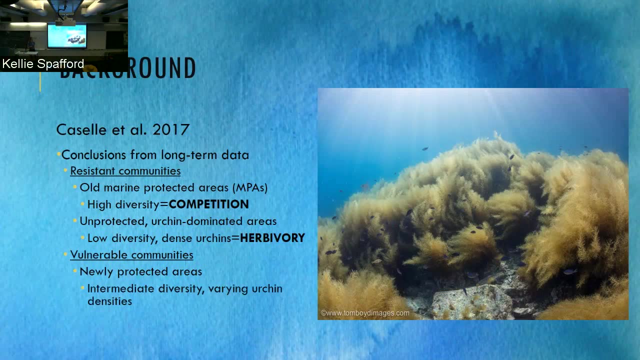 communities that had recently been protected from fishing but didn't really have a chance to develop an abundant predator population or had varying urchin levels, So neither competition or herbivory were strong enough to control Sargassum horneri there. 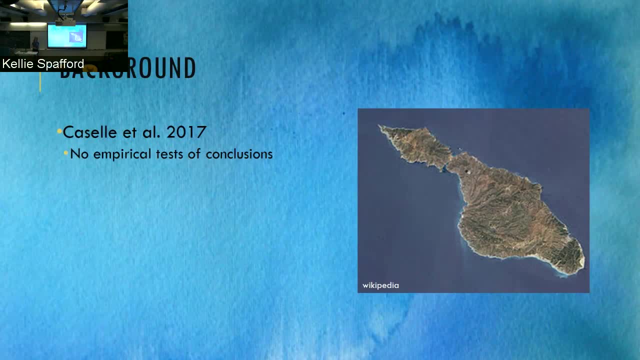 research, as I mentioned, was all derived from long-term data and there weren't any empirical test of these conclusions. Also, this was only concluded for the Northern Channel Islands and specifically Anacapa Island only. So my research specifically seeks to address whether competition in herbivory so 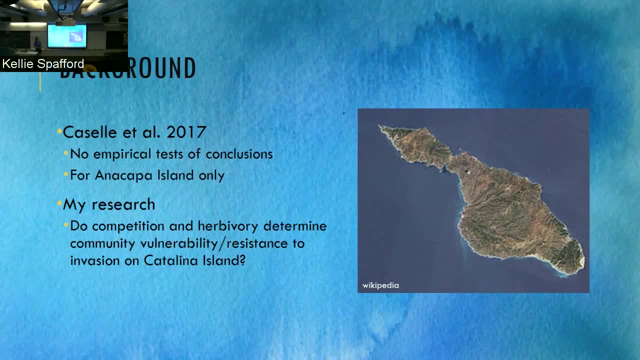 competition via algal diversity and aversion of herbivory determine community vulnerability and resistance to invasion on Catalina Island specifically, but the Southern Channel Islands in general, because the Southern Channel Islands are quite different than the Northern Channel Islands and there may be different. 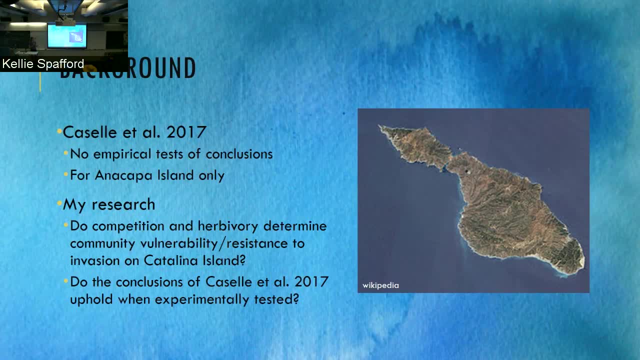 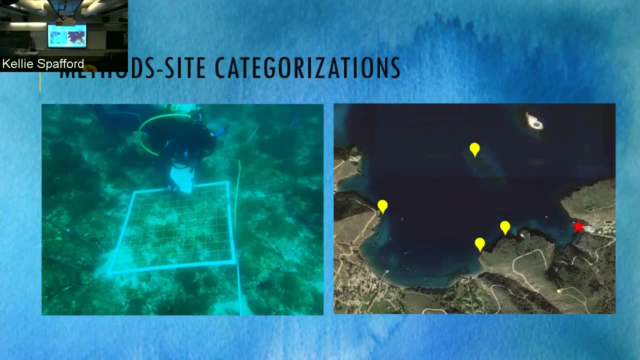 dynamics at play. And then another one of my questions is: do the conclusions of this previous research uphold when experimentally tested? So do the conclusions from the long-term data actually match what is happening in the field? So to test these questions, I first chose four field sites. The first let's see. the first one is: 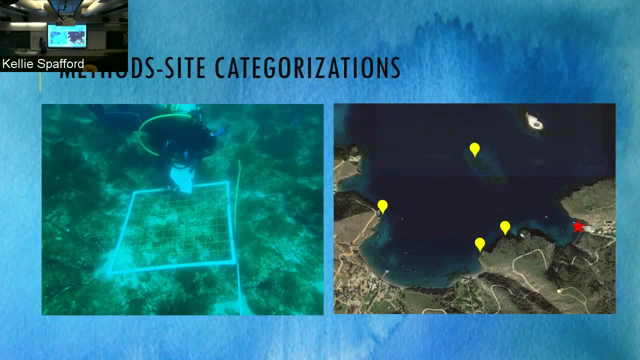 Isthmus Reef, then West Two Harbors Campground, which is by the Two Harbors Campground, and then Chalk Cliffs, which is just outside the Blue Cavern MPA, And then this red star represents where we are now at Rigley Institute. So my excellent dive team and I 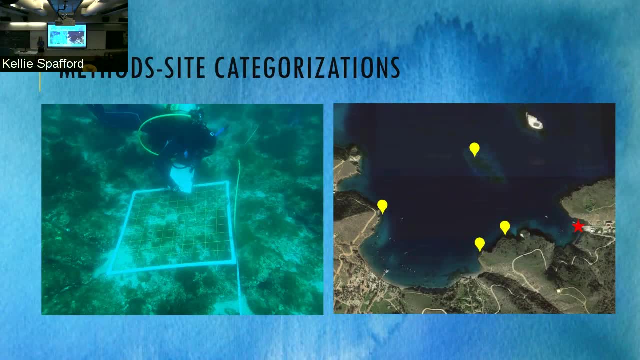 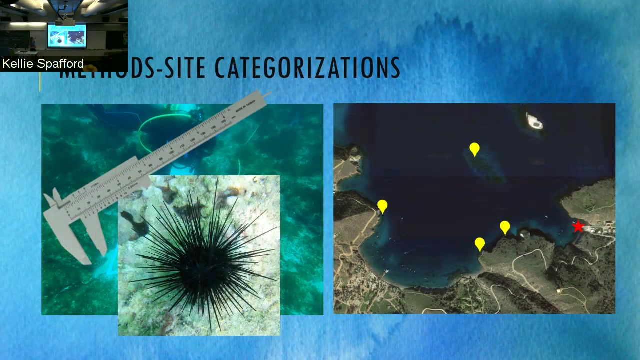 Lauren, we first conducted a bunch of quadrat surveys where we looked at algal diversity, invertebrate, different invertebrate abundances, and then also took abiotic measurements of substrate and relief types in these communities. Additionally, we also counted and ID'd the number of urchins in these sites. 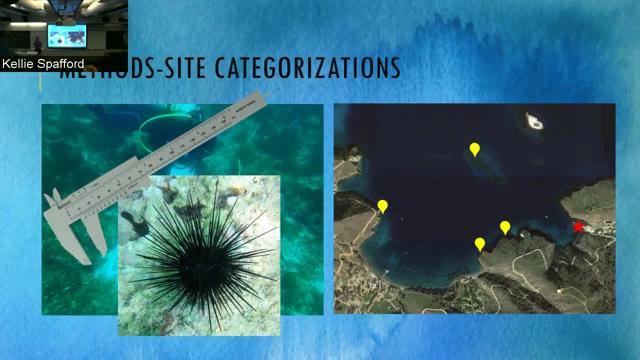 basically along a transect, and we also measured the test size of these urchins to get kind of a holistic representation of what was going on in these communities, based on the predictions by this previous research, And what we found was that there were significantly more urchins in the 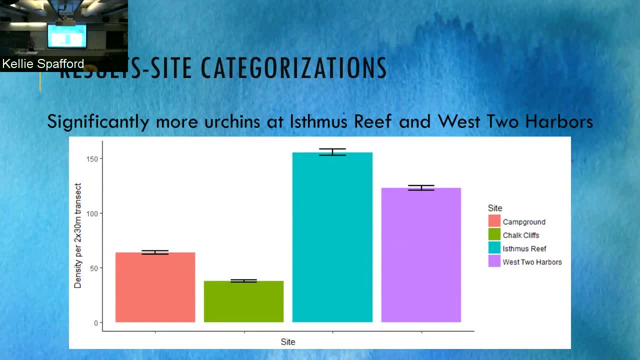 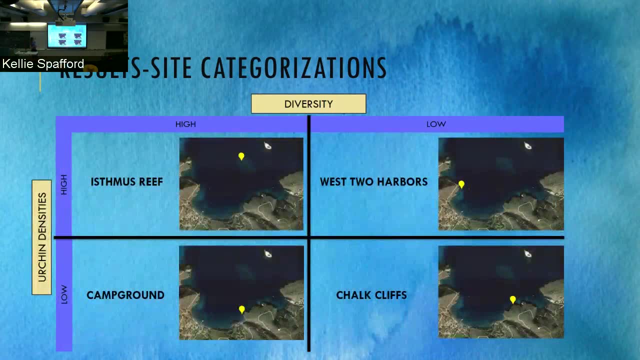 community at Isthmus Reef and West Two Harbors than the other two sites, which was perfect to test the hypothesis of herbivory as a mechanism controlling sargassum, And then for algal diversity to measure competition. we found that 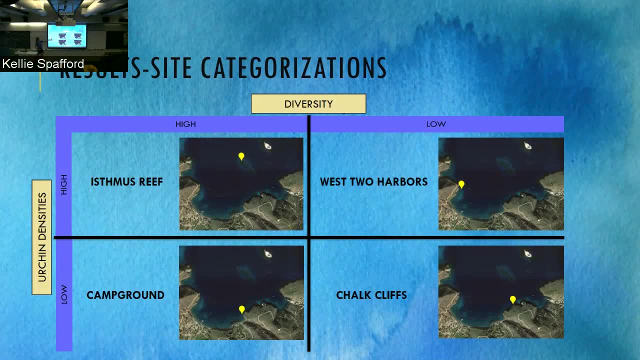 there was kind of a gradient of these sites. So Isthmus Reef had the highest diversity and also the highest, one of the highest- urchin densities there. So I predicted that this site would be most resistant to invasion because both competition via algal diversity and herbivory would be strong enough- maybe strong- to control. 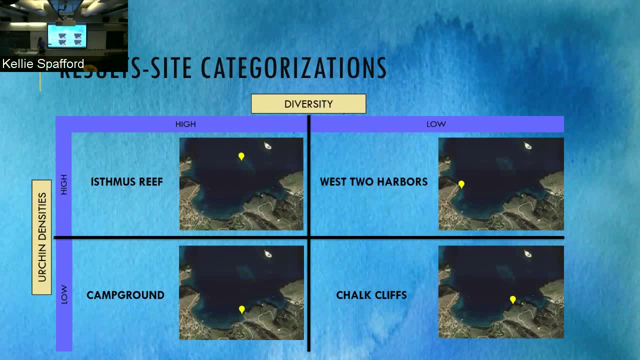 sargassum hornoid there And then Campground also had a high diversity but low urchin abundances, So potentially competition could control sargassum hornoid and not herbivory West. Two Harbors on the other hand had high urchin densities but 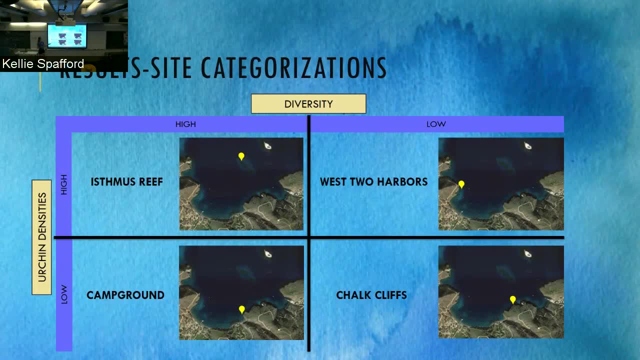 low diversity. So again, herbivory would control sargassum hornoid there potentially, but not competition. And then finally, Chalk Cliffs had both low urchin densities and also low diversity. So I predicted this site to 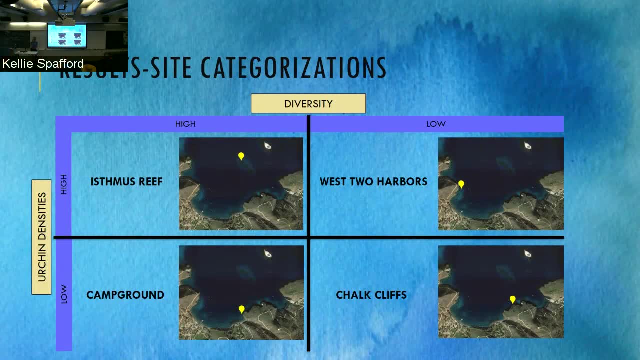 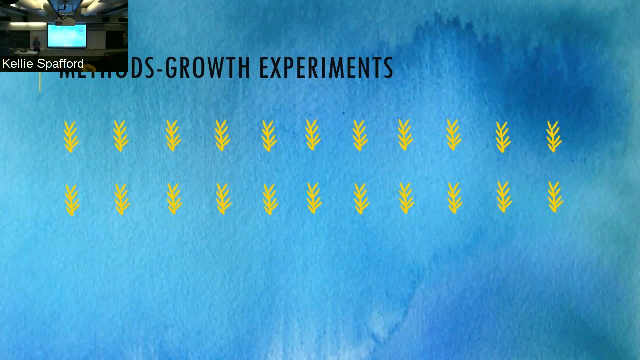 be most vulnerable to invasion because neither competition nor herbivory would be able to control it there. So then, to test these hypotheses that I had, I deployed some growth experiments, which basically consisted of me collecting a bunch of little baby sargassum, or 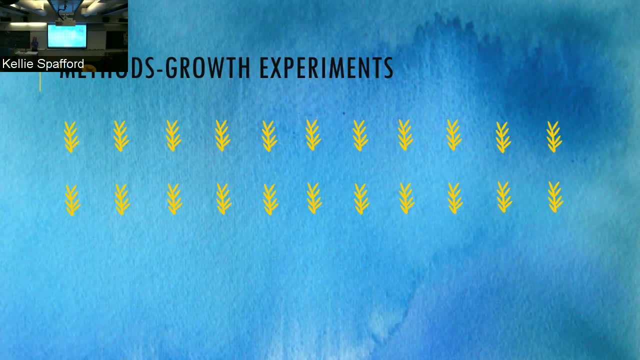 right now, most of it's in the recruit stage. so less than five centimeters in height. and then spinning all of the algae in a state-of-the-art device, a low velocity centrifuge, otherwise known as your household salad spinner. So this 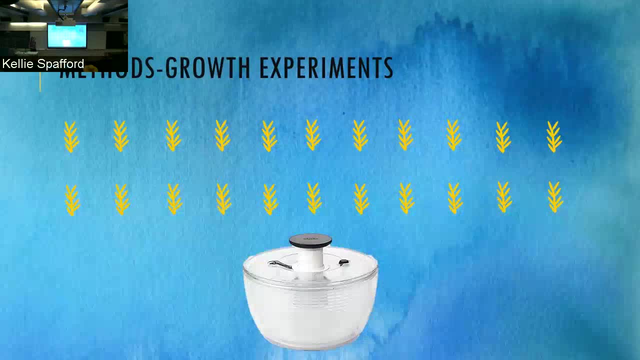 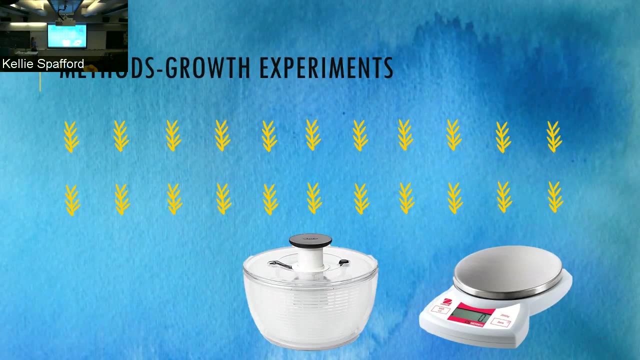 basically standardized the amount of water that's on the algae and allows us to get an equal representation of how much each algal weighs. So we would weigh the algae after we spun it down and also take maximum diameter and height measurement, And then we touched on the 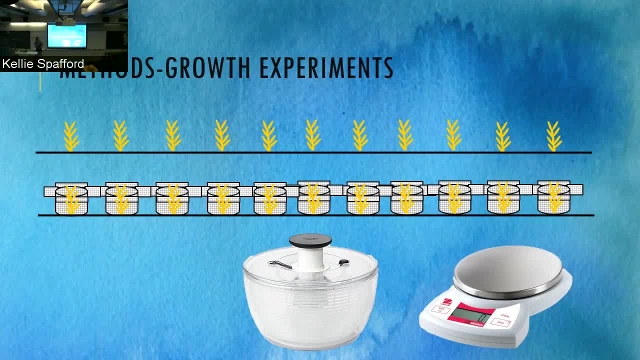 size of all of them to rope, and we caged half of them or so half of the replicates per site. So these cages are completely closed on the bottom and the sides but open at the top, And so they have these lifts at the tops that, basically, are specially designed to prevent urchin herbivory. 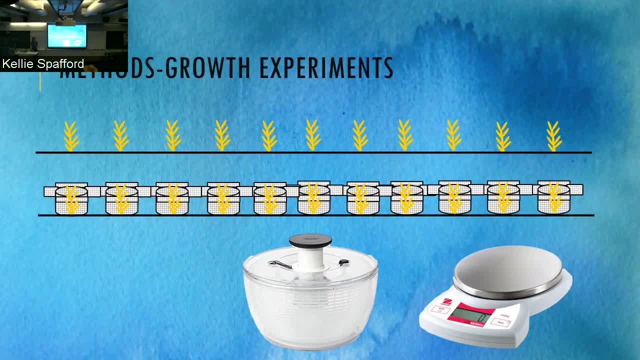 specifically but allow other types of herbivory to occur. So as the urchins climb up the sides and reach the lifts, they can't hold on anymore and they fall down. So it's been specifically designed to prevent urchin herbivory, but it seeks to address the pressure of urchin herbivory. 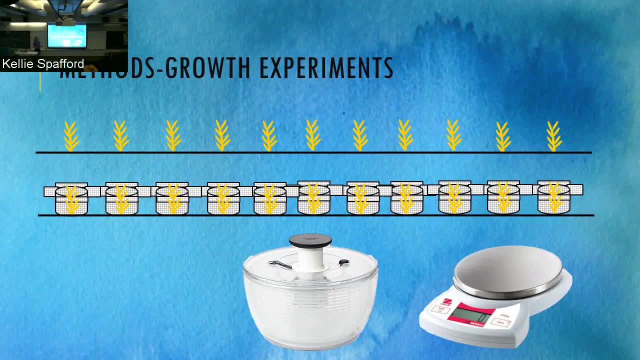 which was what was predicted to be controlling sargassum from the previous research. So then we deployed these experiments at each site and then, to make sure that environmental conditions were similar between sites, I also deployed temperature and light loggers. So after two weeks we collected everything again and re-weighed everything and measured the diameter and height again to see how much each of these. 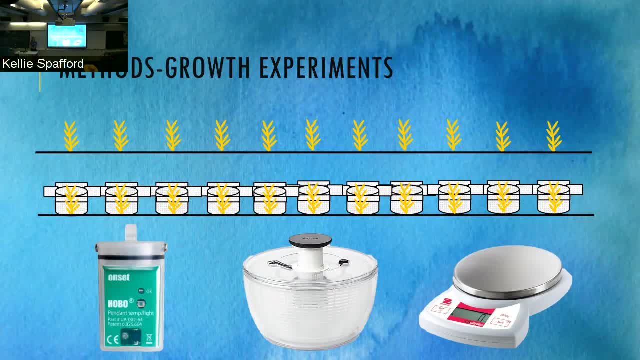 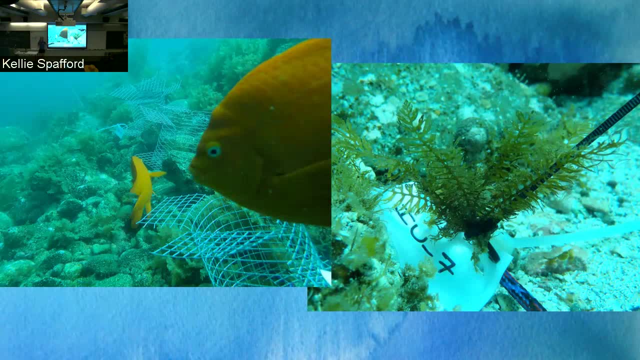 sites grew, And so these are just some pictures of my experimental units. On the right are my uncaged algae, and then on the left you can see these cages with the lifts and are like open at the top, and then also an excellent photobomb. So what I found was that herbivory and competition. 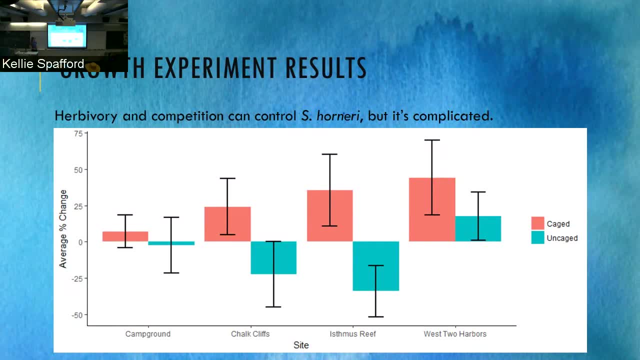 can control sargassum formeri, but it's complicated, So I'd like to start off first with um isthmus reef, which I predicted to be most resistant to invasion, And you can see that it appears that that's the case. So sargassum formeri grew the least at this site, but because there's 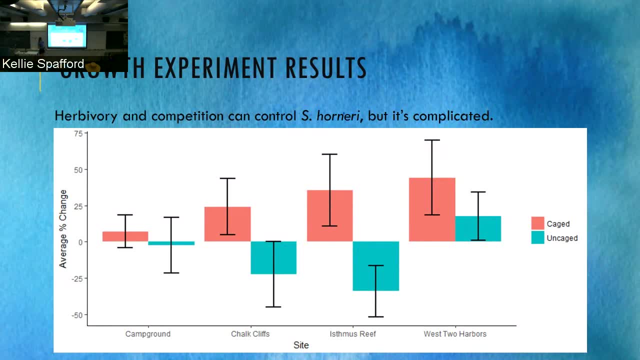 such a discrepancy between the uncaged algae and the caged control, I concluded that it was probably herbivory that was controlling it the most here, because the caged controls grew so much more than the uncaged one. And then west two harbors is interesting. I've been trying to figure out how to interpret this. 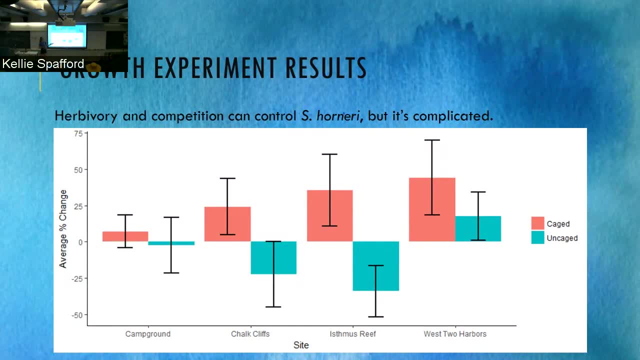 and this is my best interpretation. So, even though there were a lot of urchins at this site, this site also had the greatest amount of open space than any other site, So there's a lot of bare rock there. Urchins are known to really only graze within a certain radius of their home. 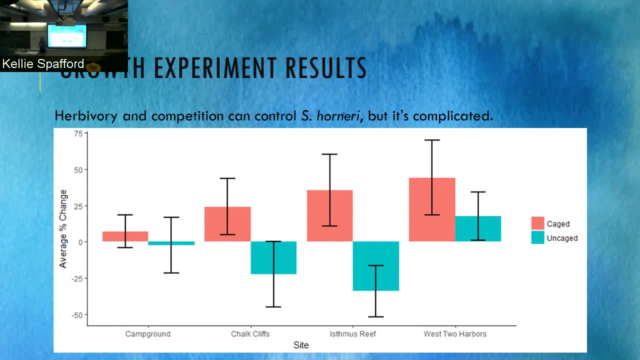 crevice. So I figured that potentially where we laid down the experiments were outside of the grazing radius of these urchins And because there wasn't a lot of other algae to compete with sargassum formeri right there, it was actually able to escape both herbivory and 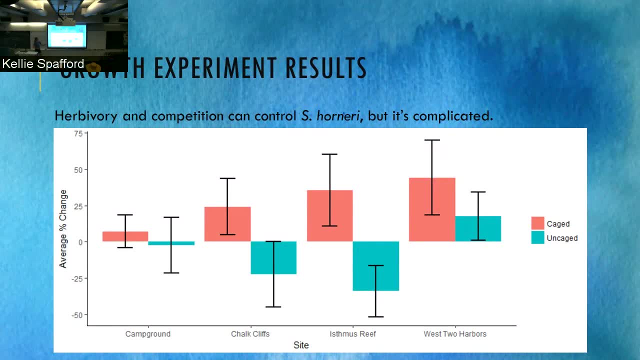 and grew the most Campground. it didn't really change that much. but Chalk Cliffs is another interesting one because I predicted that this site would be most vulnerable to invasion. So sargassum formeri would grow the most here because neither competition or herbivory were really strong. 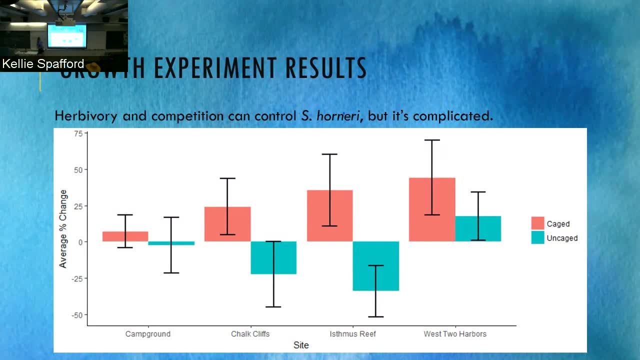 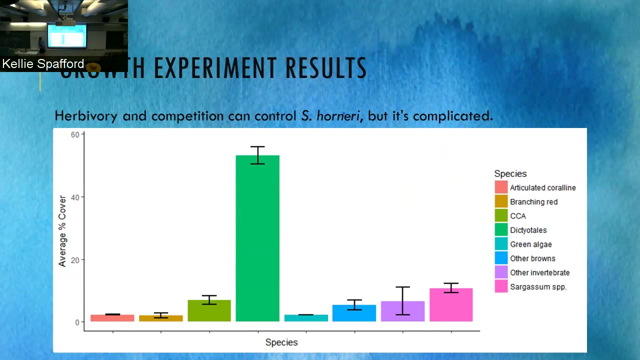 there. But what I found was that I was using algal diversity as a proxy for competition, which I now realize may not be the most reasonable way of looking at competition. So Chalk Cliffs actually has a very high percent cover of this order of algae called Dictyotales, And so Dictyotales forms. 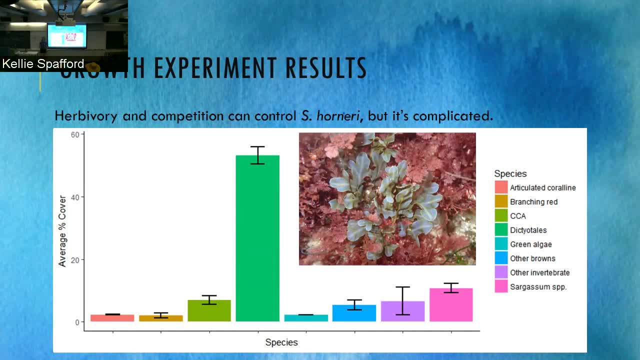 these like this dense, like kind of mat underwater, And I figured that because sargassum formeri decreased in growth so much that it was actually competing with this dense algal cover. So there's almost no open rock here at all, So it was still maybe competition that was inhibiting. 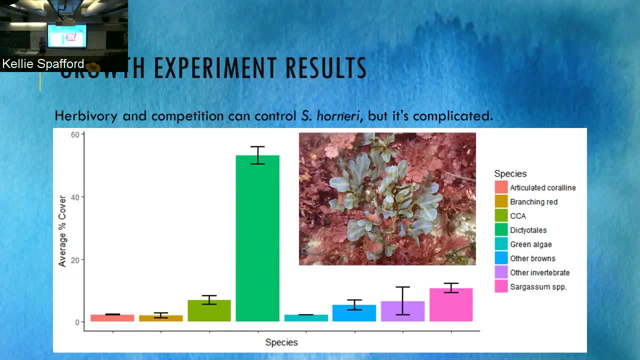 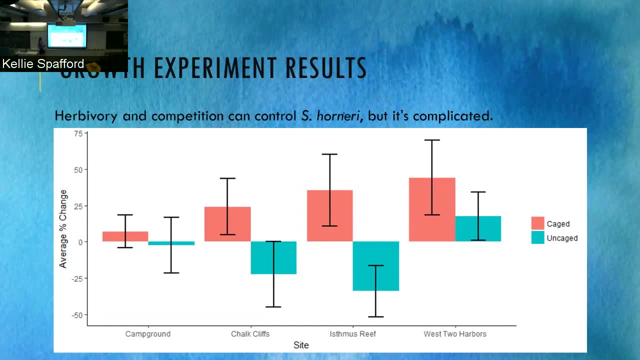 sargassum formeri here, but not so much as a function of algal diversity but mostly just the total algal percent cover at this point. But then I figured that if this was the case then the caged and the uncaged control should show a similar path growth pattern. because it wasn't. 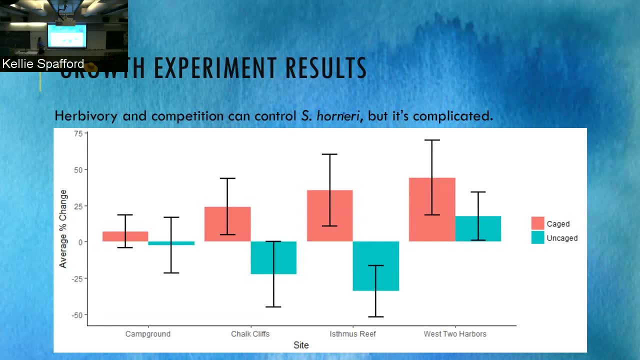 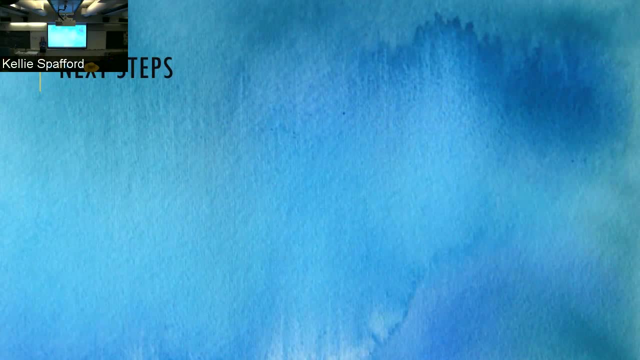 really herbivory that was controlling it here, but competition And this led me to realize that there was probably a flaw in my experiment design. So right now my cages are completely closed on the bottom And when we would put them out on the algal beds it kind of smushed all the algae. 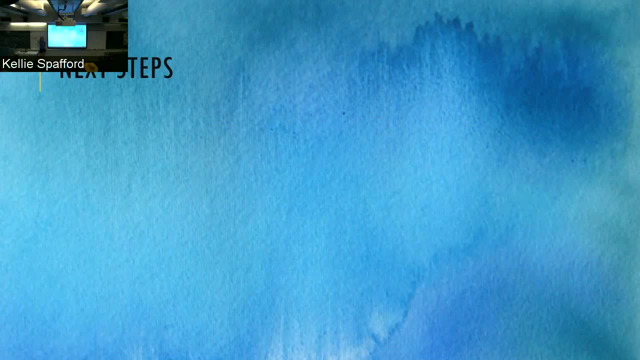 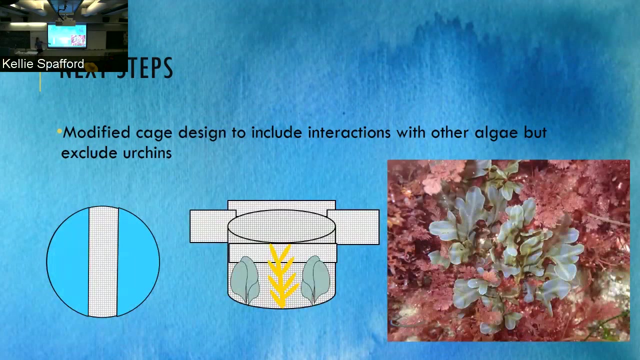 underneath it and allowed sargassum formeri in the cage to get a competitive advantage over the algae underneath it. So it had readily access to light and space that it didn't really that it wouldn't really have otherwise. So this led me to modify my cage design to be completely open on both sides of the bottom. 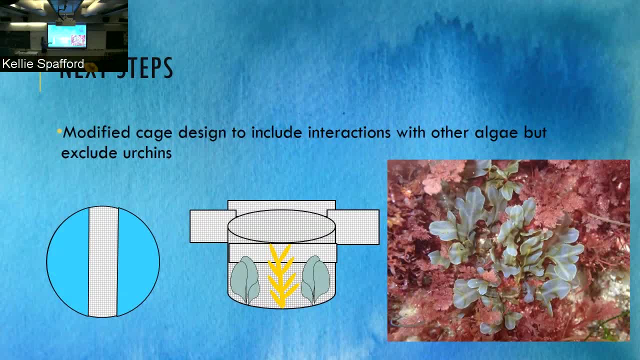 save for a small strip of cage that we would attach. we attached sargassum formeri to, So this allowed algae that was growing on the bottom to interact with sargassum formeri still, but have the cages still exclude urgent herbivory? So we have. I actually have an experiment out in. 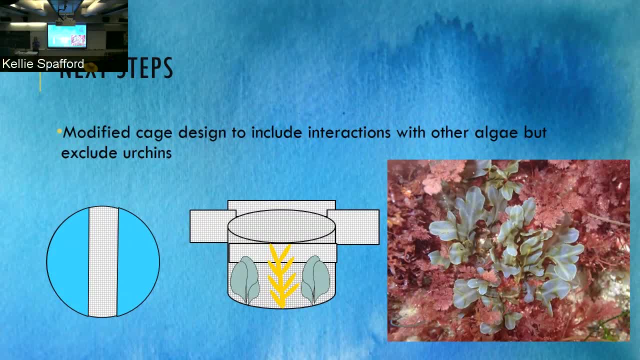 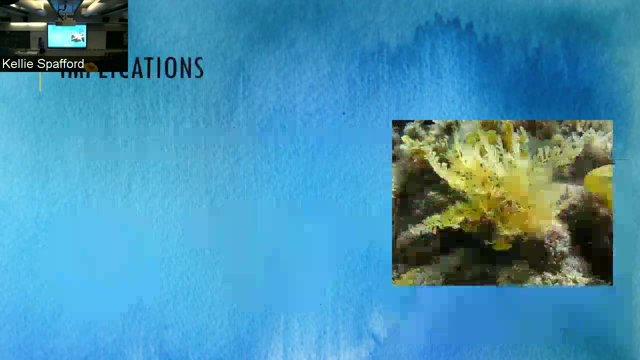 the water right now and we'll see how, what the results look like, because this will allow me to kind of get a better representation of how competition and herbivory may impact sargassum formeri at a more accurate and final resolution. So implications for this research, it's apparent. 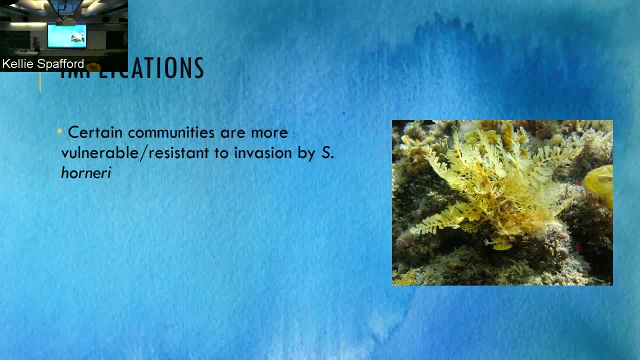 from the results of my experiment, also previous research, that certain communities are more or less resistant to invasion by sargassum formeri. Recent attempts at removals of sargassum formeri found that in the removal plots sargassum formeri was more dense than prior to removal. So it was 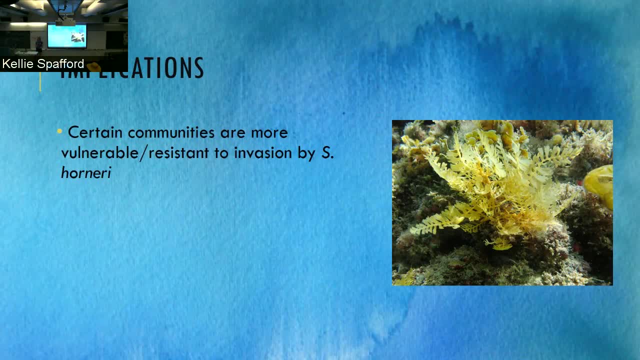 concluded that widespread eradication of sargassum formeri is likely, not feasible. but recently invaded sites before sargassum formeri is able to establish should be targets for control and removals because they haven't really had a chance to establish a strong population. So my research 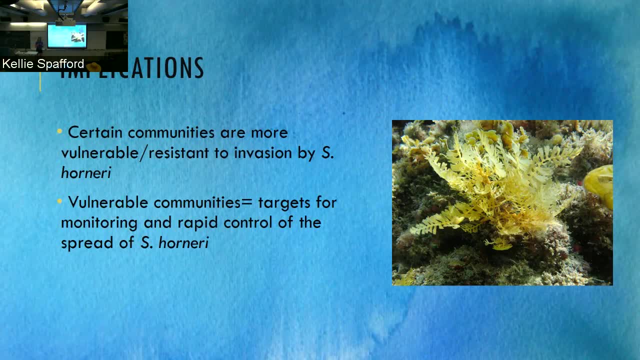 seeks to find find these vulnerable communities and then also use them as targets for rapid monitoring and rapid control for the spread of sargassum formeri. So we may not be able to fully eradicate it now, but we can control the spread And then also further understandings of these invasion. 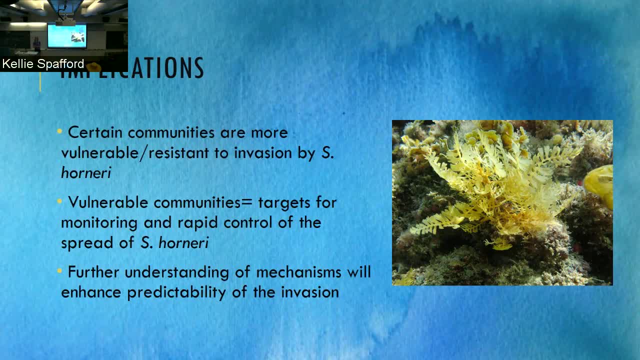 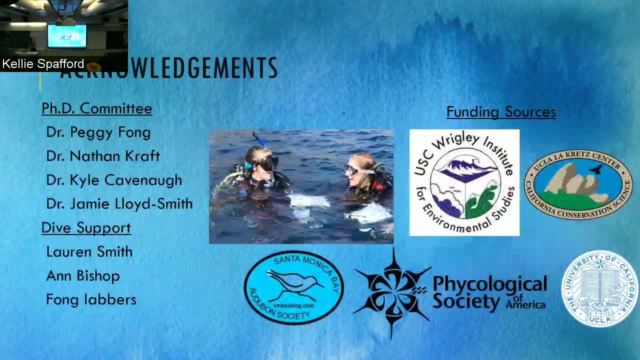 mechanisms such as competition and herbivory will enhance the predictability of the invasion. so where sargassum formeri may be. So I'd like to thank a couple people for helping out with this research: My PhD committee, particularly my advisor, Penny Fong. 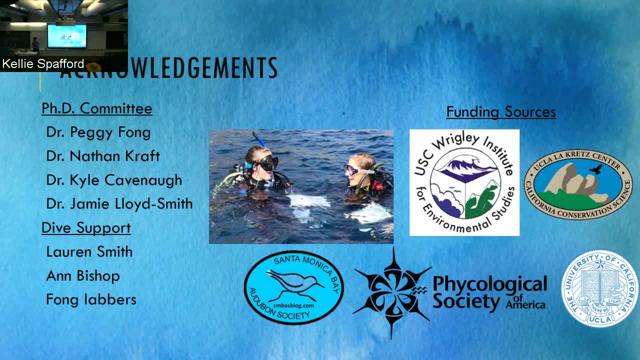 my excellent dive support, Lauren Smith, who's in the crowd here, and then also a variety of funding sources, specifically the Wrigley Institute, for giving me the amazing opportunity, for letting me come out here and do my research and also incorporating me into this wonderful community. 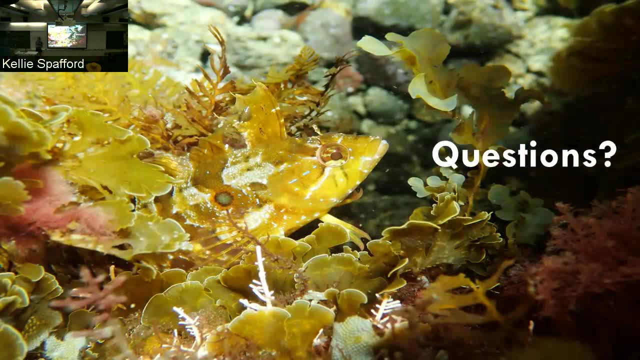 So any questions? Yeah, First of all, that's a great talk. Secondly, if you grew up in Michigan, then you know the story of the alewife and the coho salmon, I think so. In other words, the alewife was brought in by shipping and had no natural enemies. 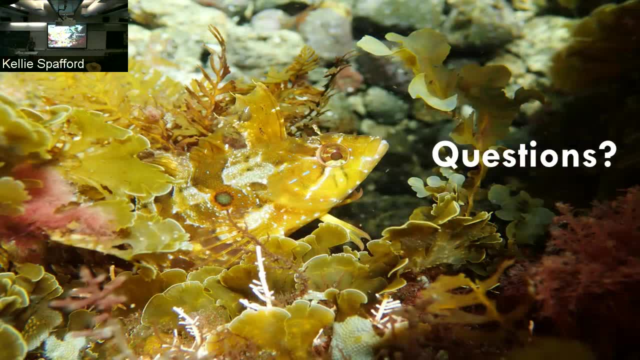 so it overtook Lake Michigan And when they would have a die off, tons and tons of dead fish would build up on the beaches. And they solved the problem by introducing coho salmon into- I know- Lake Michigan because that's where we live, on Lake Michigan. 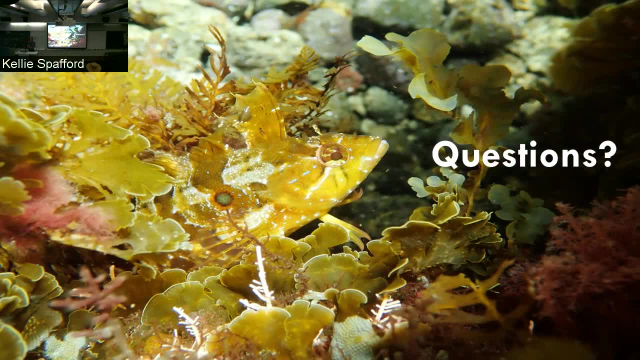 And I just wondered if there's a possible analogy here. Is there something from Korea that we would rather have in this water than to have that loves to eat this stuff? So that's an interesting question. I think there are success stories with introducing species from the native range to control the invasive and the invaded range, But a lot of. 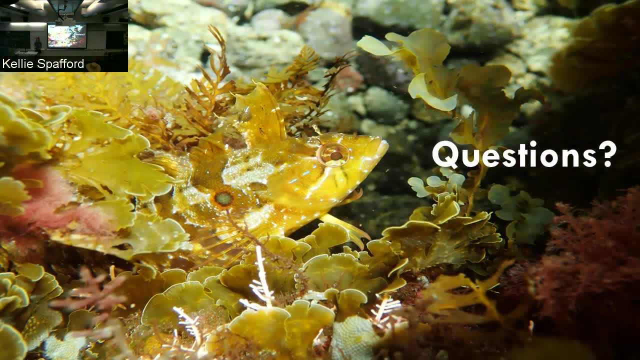 times it basically causes another introduction of an invasive species. So like, let's say, if we brought like urchins from Korea to Catalina Island to control Sargassum porneri, they may control Sargassum porneri, but they may also eat a bunch of other algae here. 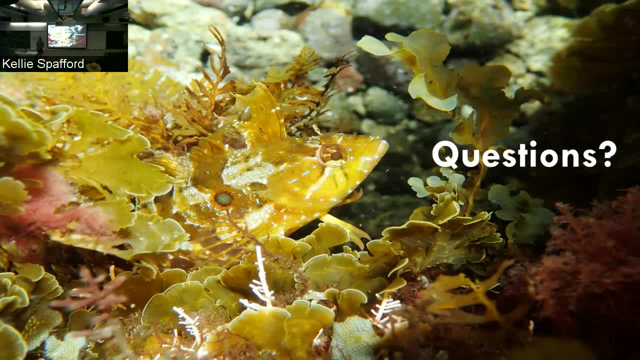 too, So they maybe become another problem. So that's an experiment, isn't it? It is, it is If it's able to be like, if we can control— It looks like there were some inland lakes that had this problem, right? 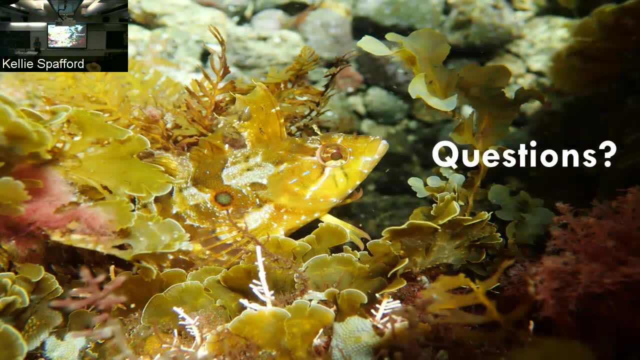 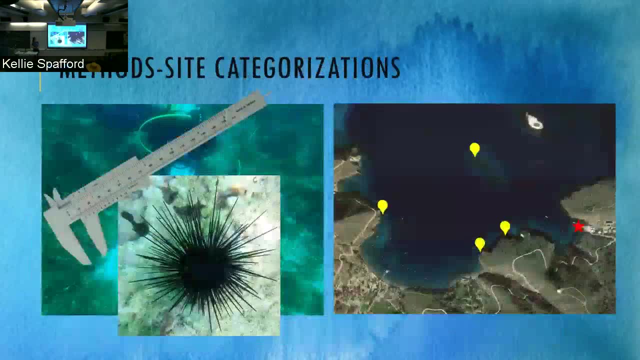 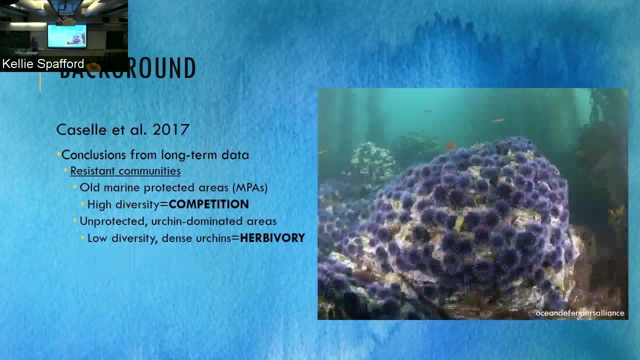 Inland lakes, Sargassum. Yeah, When you showed the map- maybe I got it wrong, but it looked like— It looked like there were some black dots of infection inland, not just in the ocean. So it is. it's a marine algae, so it shouldn't be able to go inland, But let's see—. 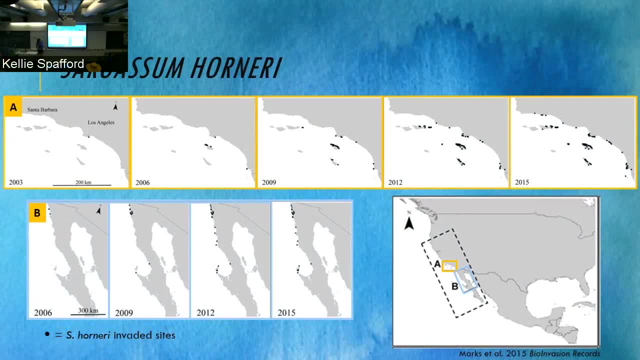 It needs saltwater. Right, Yeah, so this is— The White's Ocean. Yeah, okay, you're right, I misread that. So you'd have to take one isolated area and run an experiment. Yeah, I think it would have to be very carefully monitored They. 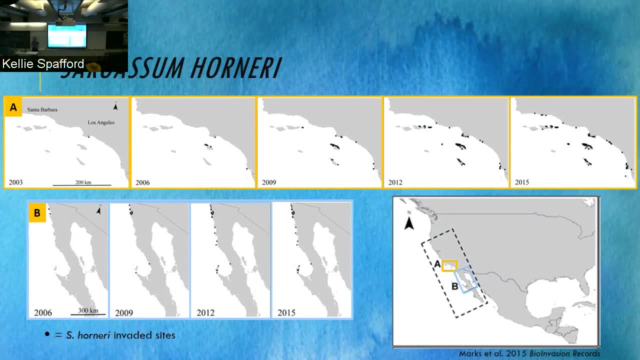 may be like a small scale first, But I think, yeah, like that's an example of a success story, But a lot of the times it just— It does end up introducing like another invasive species Causes like two problems rather than one. We love the salmon. 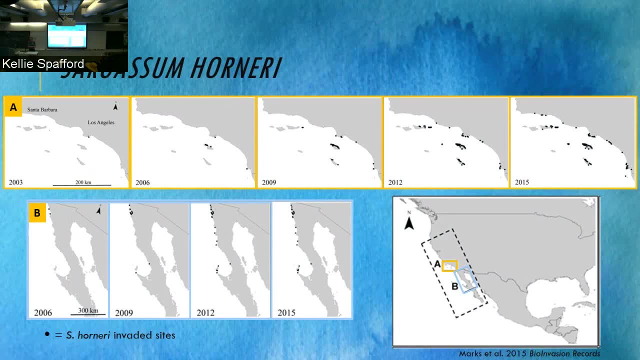 What We love. the salmon boy. I got a question And you might have already covered this and I'm probably going to butcher the question, but you mentioned most susceptible areas are newly protected regions, So like if you have any kind. 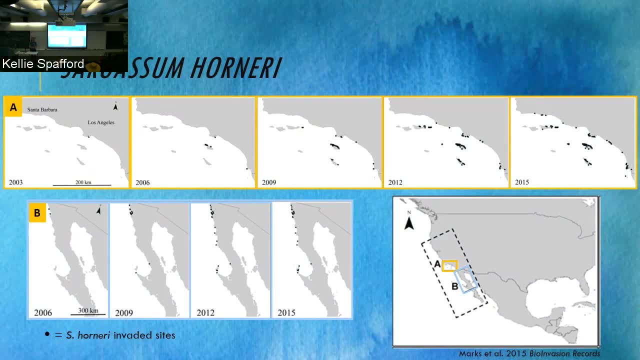 of natural disaster. you have like primary, secondary succession, like: is there evidence to show that after a time of being protected, that the ecosystems will kind of balance themselves out and native species will move back in and kind of correct itself? 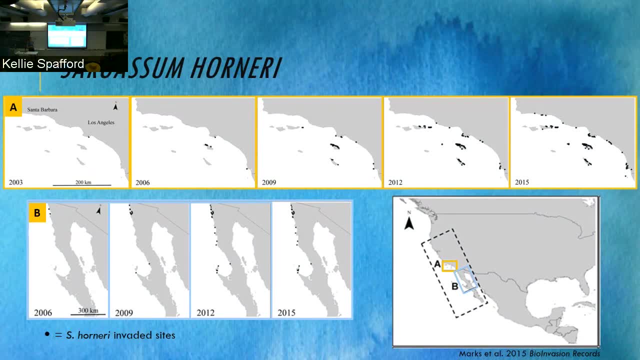 As far as the invaded areas, Yeah, So I think it's hard to say. It could be that maybe, as water is cool, so it's hypothesized, it did so well because of the El Nino on the warm water, So like potentially best case scenario. 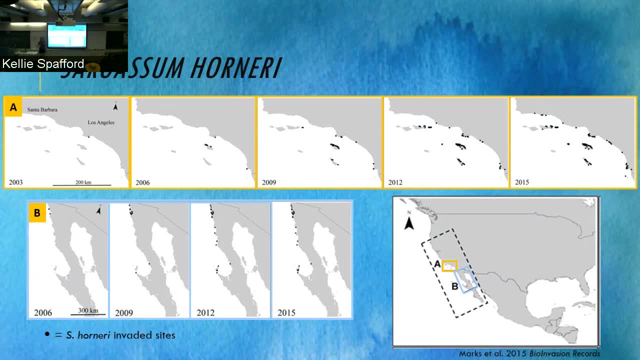 as water's cool Sargassum pornoid doesn't do as well, and the native community kind of bounces back and restores itself to its natural state. Another hypothesis is that these Sargassum pornoid-invaded areas are unfortunately basically an alternative stable state, So they are there to stay. 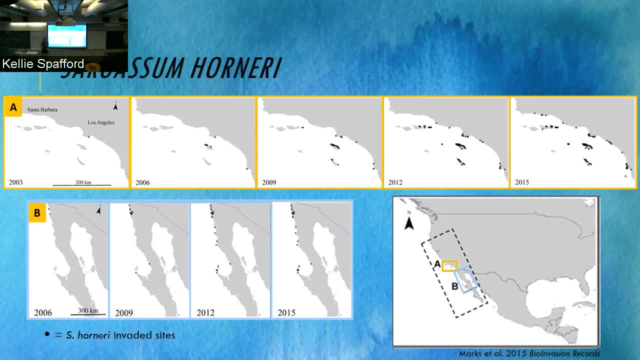 and that's what the community's going to look like for now and for the rest of the community. So I don't know… I can't really say. I hope that the community will bounce back when protection kind of is established and is able to, I guess. 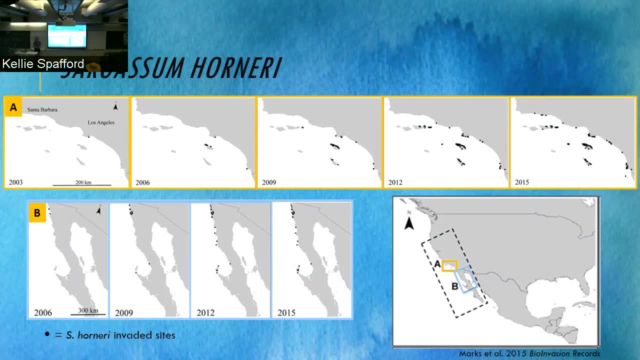 kind of create a diverse community more. But it's hard to say, Yeah, This, are you telling this to your research on the abalone? So kind of well, not really. I think like they all have an underlying conservation. 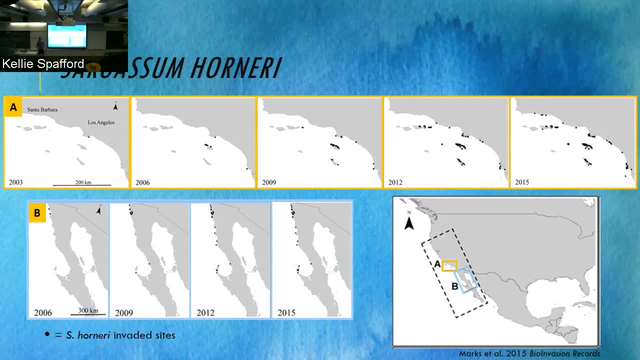 thing to say: Yeah it, but I kind of stepped away from the abalone. Potentially it would be interesting to look at maybe how sargassum frontera is impacting the abalone populations on Catalina. But yeah, I haven't really sought that path yet. Have you researched on the water temperatures as to what's the lowest that they could survive at? So there has been some research in the lab. I think it's some research in the state. have been looking at the temperature tolerances of sargassum frontera And then my lab mate. 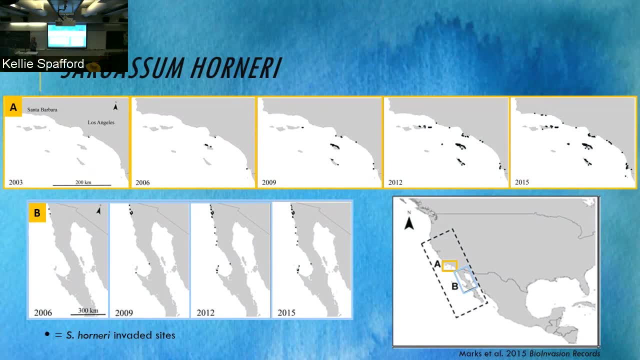 Lauren is actually looking at how competitive interactions between sargassum frontera and native algae change with different temperatures. So yeah, Because right now we're going through a heat wave for the last 10 years or so- that if we reverse and go to cold water it would solve the problem. 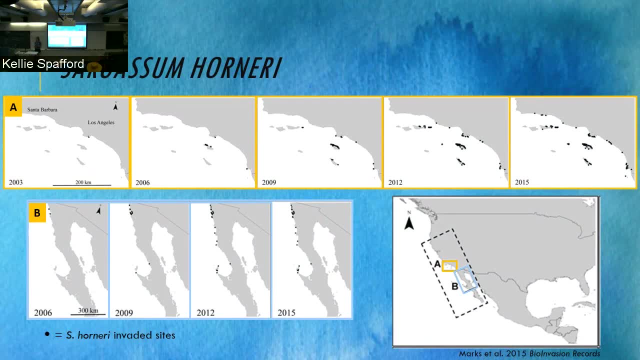 Yeah, So there's also some insight that you can take from. So this algae in its native range is actually heavily cultivated for agriculture And so there's a lot of kind of physiology data out there for this algae as far as temperature tolerances. But I would assume that it kind of matches what's happening here, but it could be different. So, yeah, What were some of the thoughts on how it found its way over here? Has it been like ties and currents, or is it like zebra mussels, like ballast water, like through human? I think it's mostly most likely human transport. 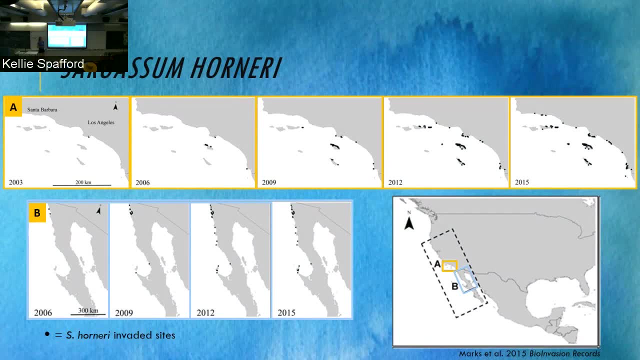 So like these large shipping crates, I don't know if it can survive very well in ballast water because it's kind of like a low light environment, but maybe like attaching to like boat hulls and coming over. There is evidence or, I guess, like how it spread throughout the Channel Islands and 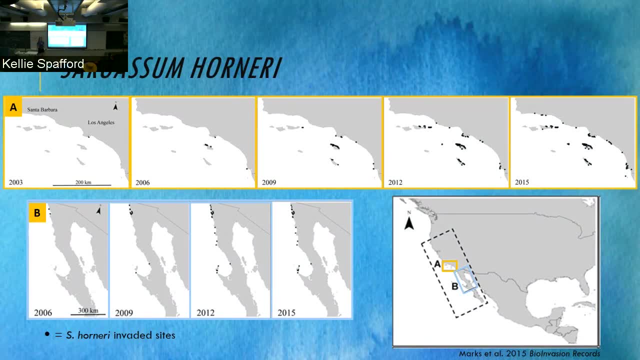 Baja could be either like Recreational vessels or because it's able to float long distances and kind of disperse its germlings. it could just be like it's becoming detached and floating with the currents and spreading that way too. So Yeah, Is this similar to Calerpa? So it kind of is Calerpa, at least in California I think, started to invade San Francisco Bay. but they really recognized its potency from how it invaded the Mediterranean and so they really like rapidly controlled it there, I think because Sargassum horneri wasn't 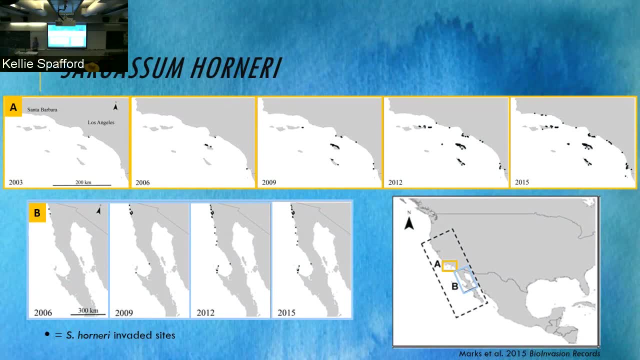 really recognized as an invasive, like right off the bat. it kind of like spread unknowingly until it kind of became too much of a problem that was really controlled. But yeah, so Calerpa is like also another invasive algae, Yeah, Yeah. 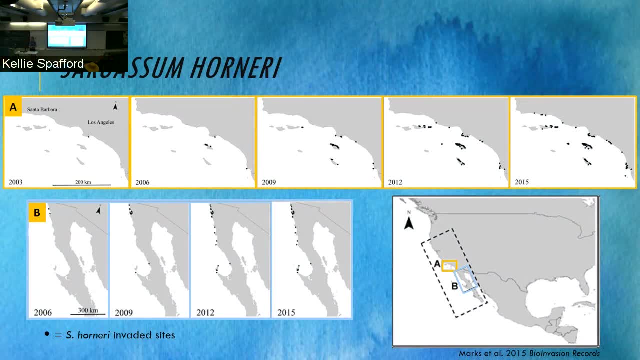 Is the algae actually going to create a large problem if they continue growing? So even though- yeah, even though- it invaded in 2003, it really only started to filth rate like pretty relatively recently. So unfortunately, there are still a lot of unknowns about how it's. 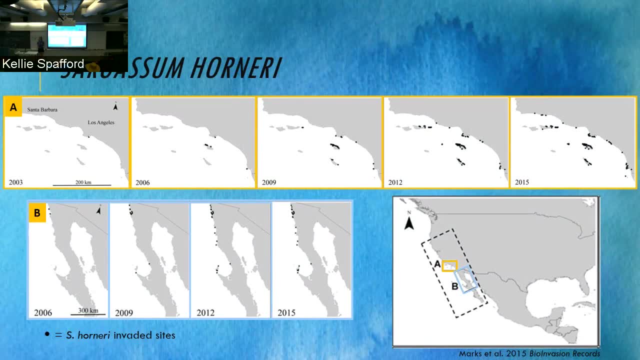 impacting the environment. but there was a study that just I think was published this month or last month that found that the kelp bass recruitment was actually significantly inhibited by the presence of algae, Or this algae as opposed to the native giant kelp. So that's one of the impacts of Sargassum. It's also hypothesized, which is 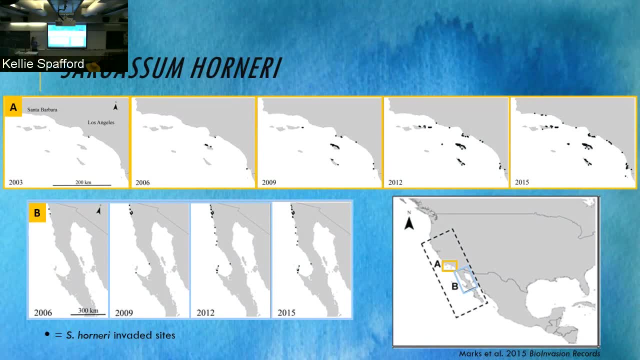 another aspect of my research that I haven't gotten to yet, but basically looking at how Sargassum horneri may be inhibiting giant kelp recruitment by taking over the space and holding that space. So that's another potential impact, but unfortunately there's not a lot of like published data. 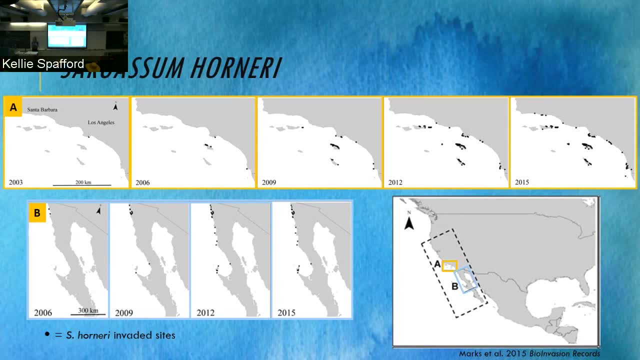 So that's another potential impact, but unfortunately there's not a lot of like published data or literature as far as like how it's impacting, but a lot of the problems. Thank you so much, Emily.